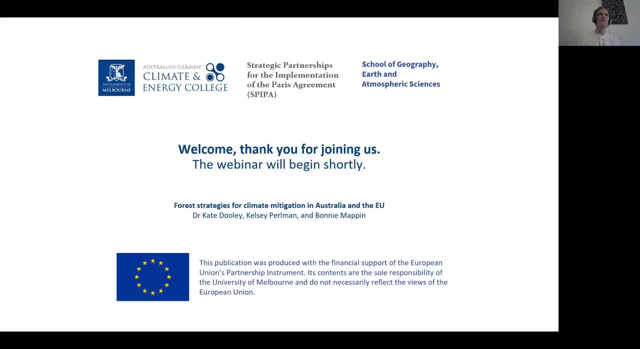 and the moderators, Kate and Angela, will kind of ask you to unmute yourself and ask the question in person if you want. that's the kind of engaging way of doing it, but it's also a lot of fun and we'll be moving through that. and we'll take a series of questions and the moderators, Kate and Angela, will kind of ask you to unmute yourself and ask the question in person if you want. that's the kind of engaging way of doing it, but it's a great thing to do and we're looking forward to answering your questions. 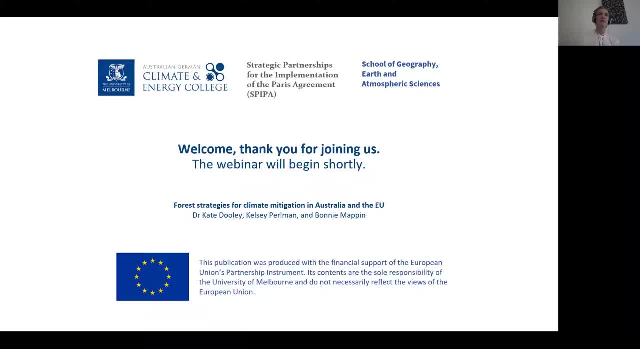 way of doing it. If you don't either ask the question anonymously or, if you'd prefer, we can read the question out for you, And there's also going to be a survey of information that GIZ, our supporting agency, would like to collect about the way these seminars work, so we'd be delighted. 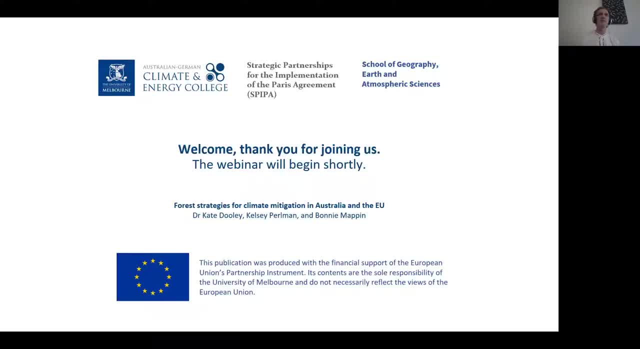 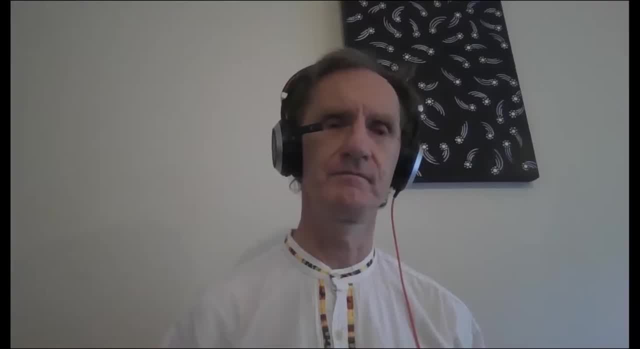 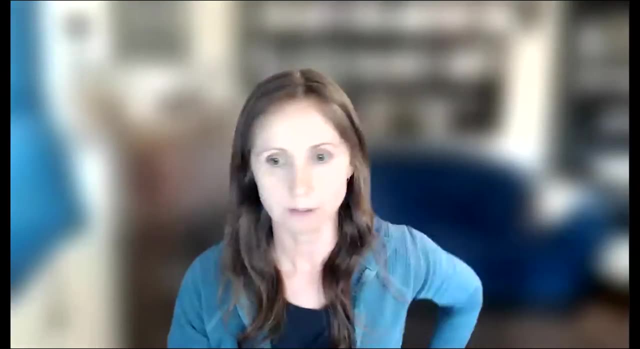 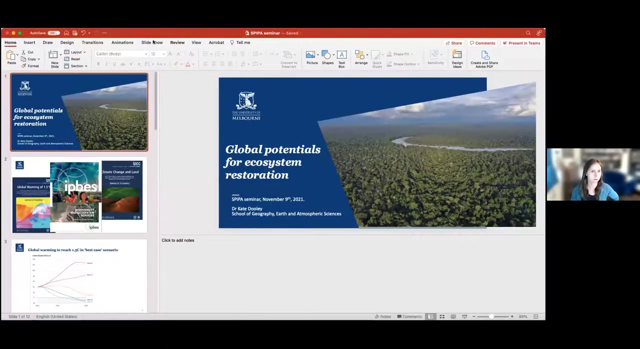 if you could fill those in for us. So I'll put myself on mute and off video and hand over to Kate, who I think is going to get us started. Yeah, thanks very much, Peter for that. I'll just turn my screen, which always takes a second, and start the presentation. 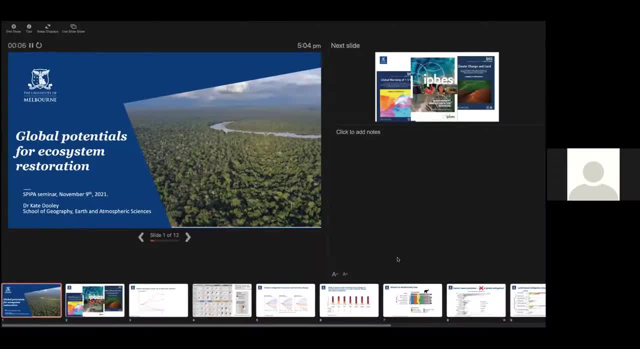 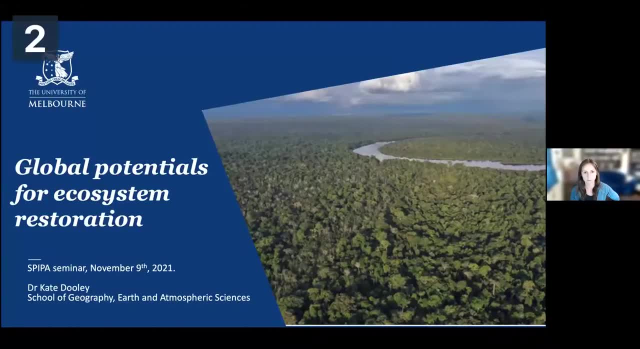 Okay, so you should be able to all see my presentation now, Okay. so yes, as Peter said, we're going to talk about land-based mitigation, but in particular, the other contributions from land to biodiversity and ecosystem, services and food security. And so my what I'm going to do. 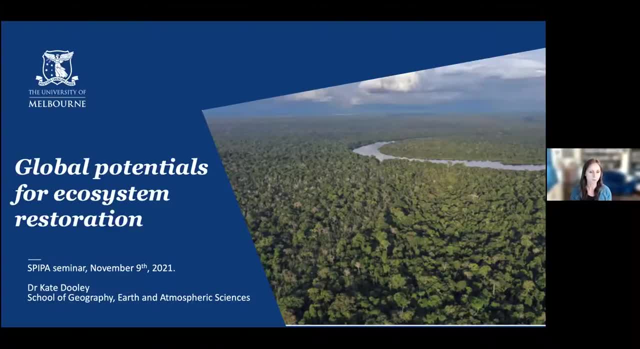 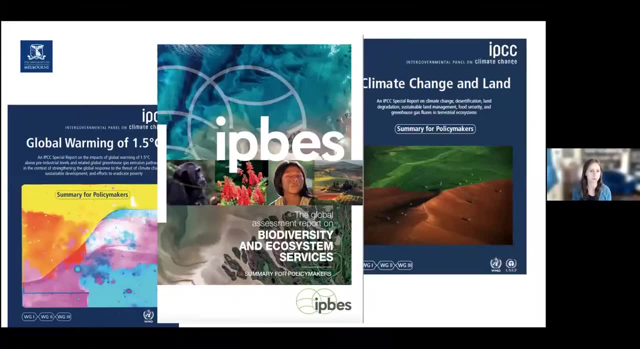 here is just give a very brief overview of um why there is so much interest really in in land-based mitigation at the moment. we hear a lot about nature-based solutions and there's a lot of focus on land, even at the cop right now- probably more focus on land than on ending fossil fuel. 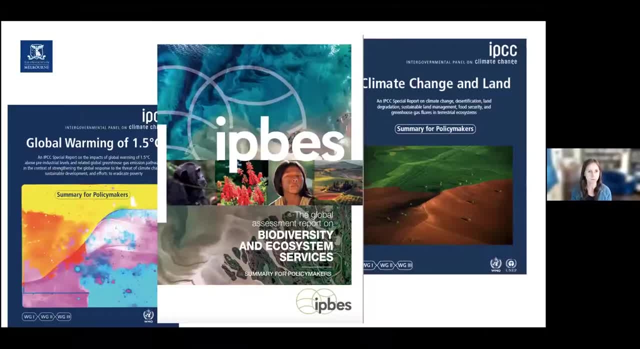 emissions. so i want to give a very brief overview on context of where this conversation has come from and what the role of land really is or should be in climate mitigation, and then i'll hand over to um kelsey and then bonnie, who are going to talk more specifically about land mitigation. 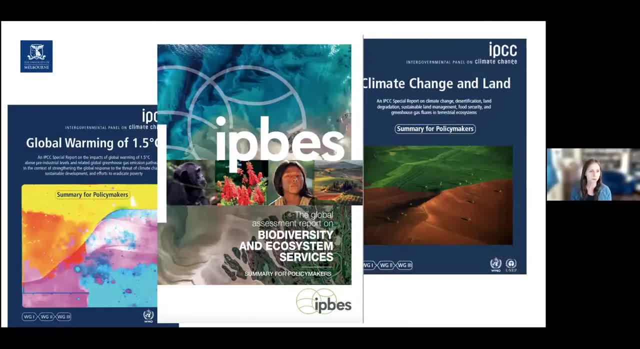 policies in in the eu and in australia. so on the slide here i have um some recent scientific reports. i'm sure everyone's probably very familiar with these. i'm flagging these up because, um, because this, obviously the science is not in doubt on climate change, but we also have so. 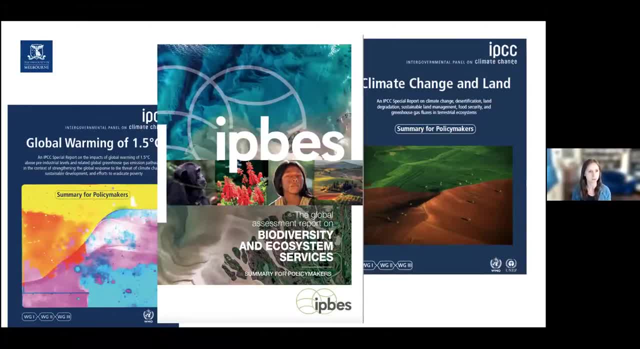 much scientific information now on the biodiversity crisis, the scale of that crisis, land degradation and um the problems ensuing from that, and also, uh, how these three things um climate change, biodiversity and and land degradation interact and contribute to each other. so the rest of the presentation, i'm going to be drawing a lot from these three reports and there's some interesting. 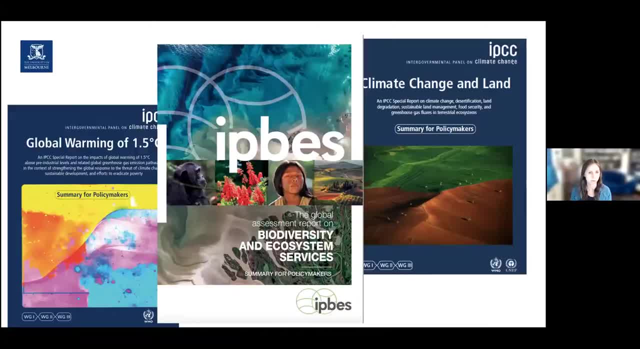 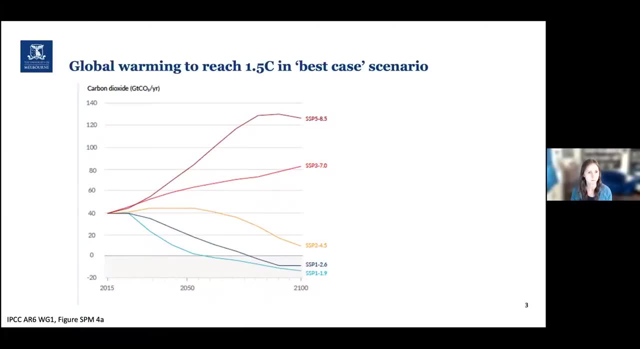 implications when we start to look at the interactions between these reports that i don't think are always brought out in in conversations around land-based mitigation. so firstly, in terms of climate change, this is actually not from the ipcc 1.5, which i showed the mitigation pathways haven't. 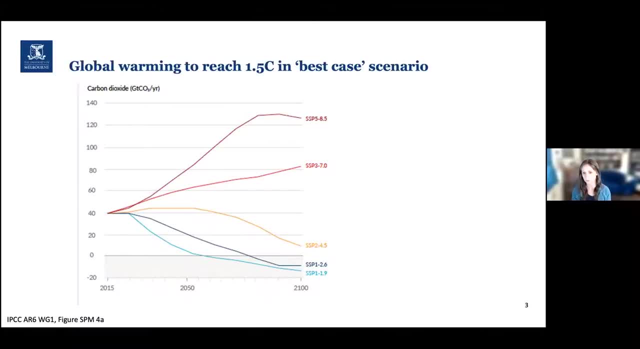 been updated yet properly, but from the ar6 working group, one report that was released a few months ago, we know that well it. there's a lot more certainty that climate, that global warming is going to reach 1.5 degrees with peak warming between 2030 and 2052. if it increases, if warming 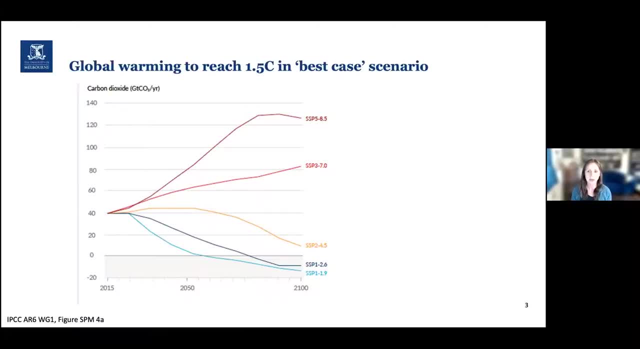 continues at the current rate or continues to increase at the current rate to the current rate, it means that there's going to be a lot more uncertainty, and so that's interesting, and what i want to show you about this slide showing um different levels of warming under different future development and mitigation scenarios is that in the cases where 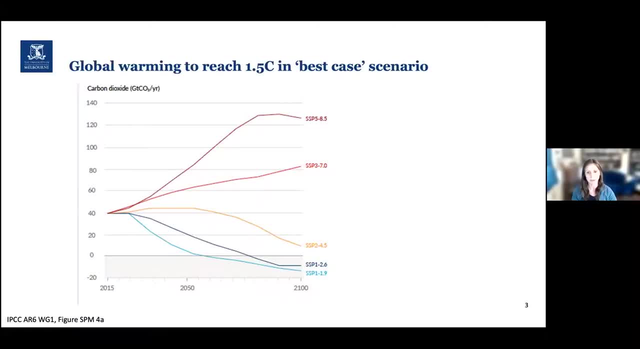 we keep um warming by the end of the century to below two degrees and below 1.5 degrees. these are the bottom two scenarios. emissions actually go negative. so this is um what these are, the at some scale. there's quite a wide range of scales in the 1.5 c report from 2018, so we 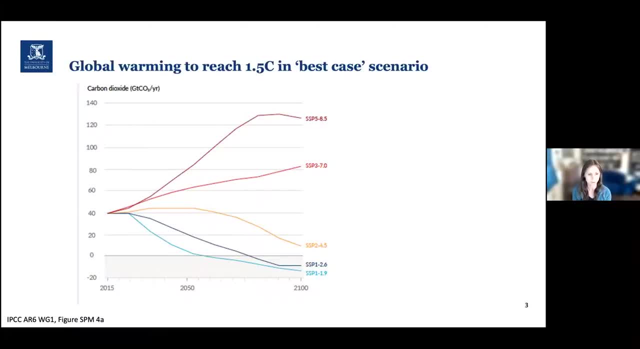 need carbon dioxide removal at some scale to keep warming below two degrees, and certainly for 1.5 degrees. and so while we now we have a crisis of biodiversity and land degradation, forests and other ecosystems are being discussed primarily in terms of their potential contribution to climate. 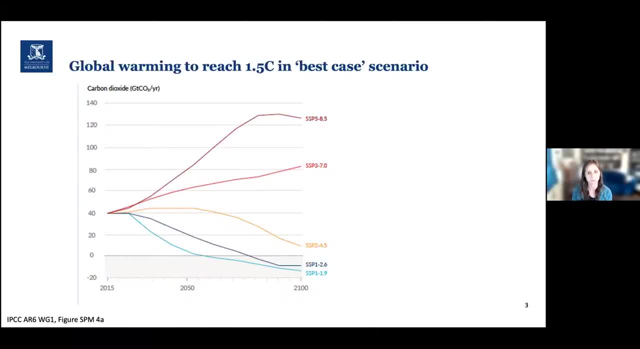 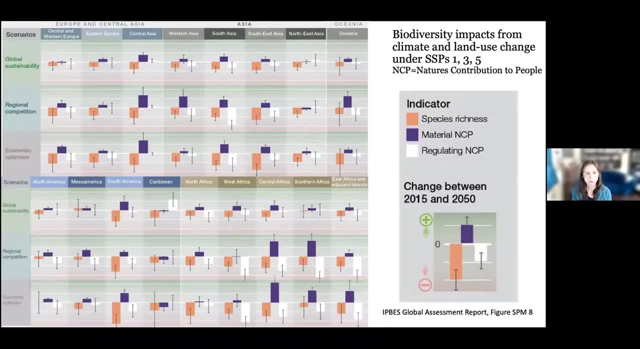 mitigation in that context of removing carbon dioxide from the atmosphere, which is needed for those low mitigation pathways. so this graph- very simple, intuitive, I'm sure it's immediately apparent what it's showing you. I'm sorry there's not a better graph communicating this finding. this is from the IPBES global assessment report from 2019 and it's assessed three of those. 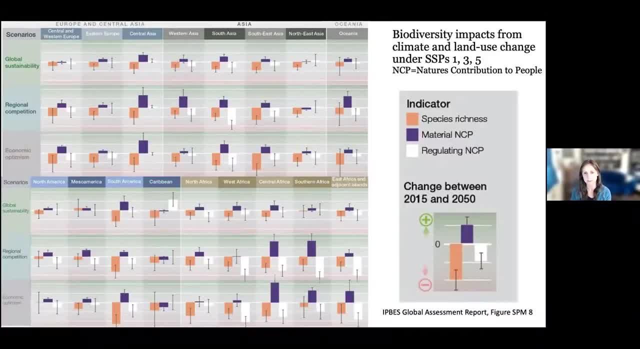 mitigation pathways I just showed you from the IPCC: SSP 1, 3 and 5. so the SSPs are the shared socioeconomic pathways. they're different developmental futures. so SSP 5 is the fossil fuel driven future. perhaps very quickly on the previous slide, it's the higher temperature outcomes from that. and then SSP 1 right down. 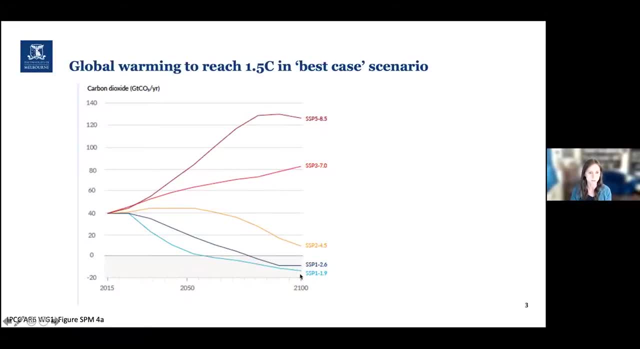 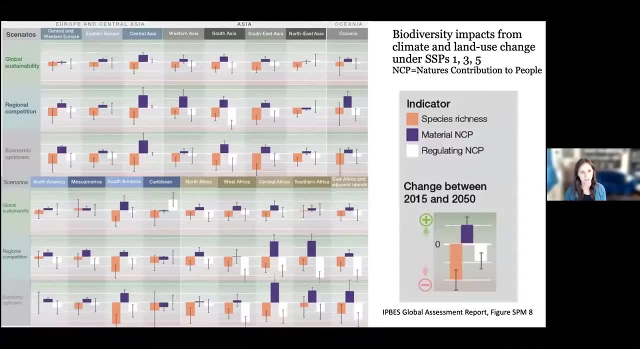 here is a sustainable, a more sustainable future characterized by equality and sustainable food and land use production systems in particular, and reduced fossil fuel emissions. so, under all of these SSPs- whether it's SSP 1, the best case scenario, or SSP 5, kind of one of the worst cases- what the IPBES found when they examine, 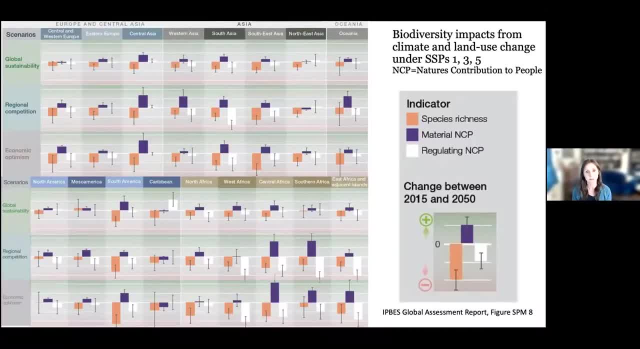 them, for the mitigation impact on biodiversity is that all climate mitigation scenarios under the SSP framework negatively impact biodiversity. so this is, in terms of what it's showing is species richness and a key measurement of biodiversity and regulating nature, regulating nature's contribution to people, which is more simply was previously known as 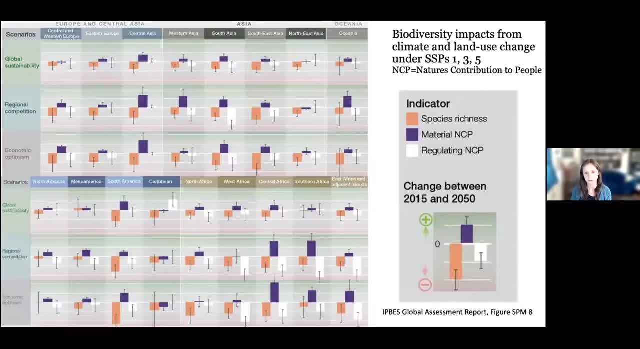 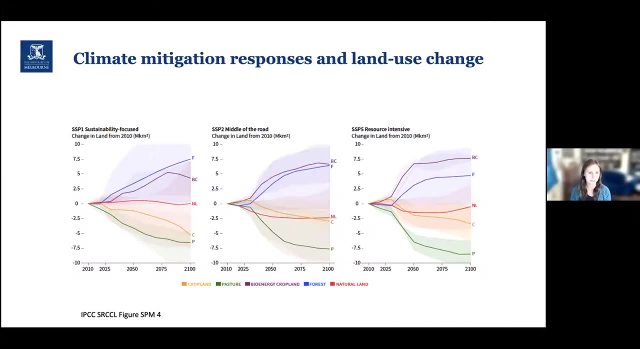 ecosystem services, so negative impact on ecosystem services that regulate climate. um so why is that? why a climate mitigation scenario is having a negative impact on biodiversity? so this is due to these scenarios relying heavily on land, specifically um afforestation or reforestation, expansion of forests and 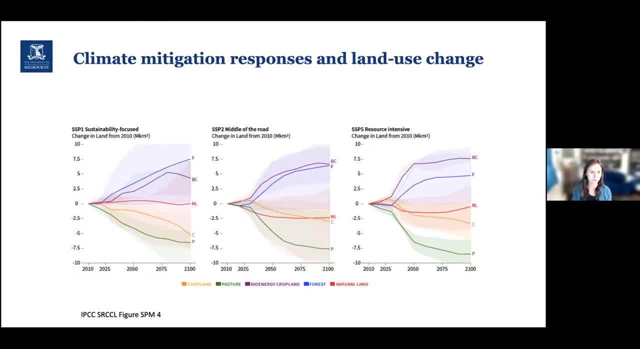 Bioenergy with carbon capture and storage to achieve that carbon dioxide removal. so for those emissions to go, negative climate mitigation scenarios are relying on land and this is from the IPCC special report on land from 2019 and it shows an increase in Bioenergy crops across all. 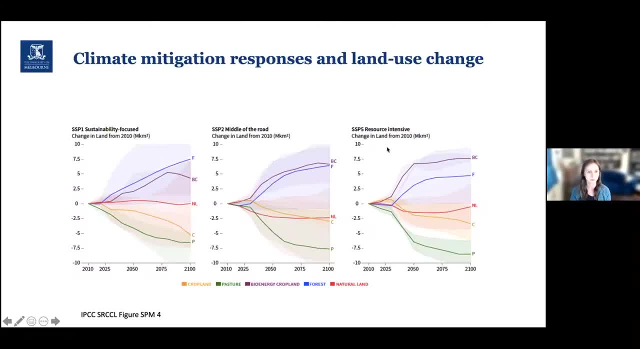 scenarios again. this is: this is comparing SSP1,, 2, and 5, so similar to the previous comparison, And we see a decrease in pasture land, a decrease in croplands for food, a decrease in natural land in all scenarios. 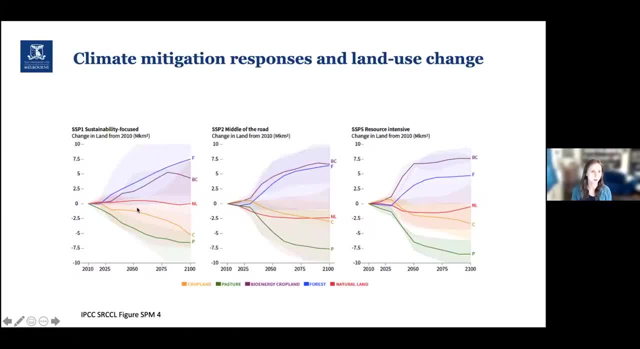 perhaps less so in SSP1.. So the point here is that in all scenarios, even the more sustainable version of future climate mitigation, there is significant levels of land use change, Really significant levels of land use change. a million extra hectares of bioenergy crops. 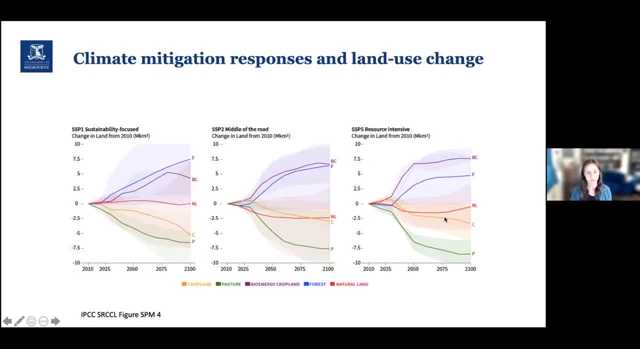 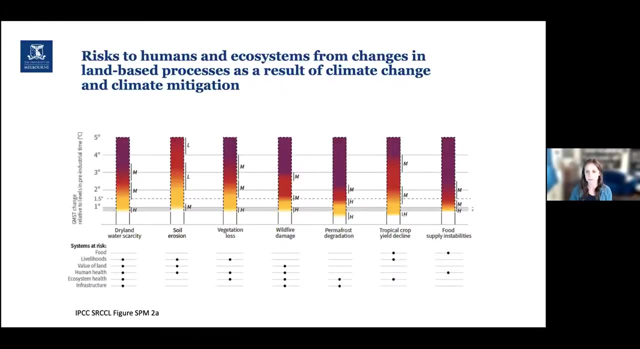 in the worst case scenario, Extra increase in forest, but these are often forest plantations. So it's this land use change that is driving the impacts on biodiversity And this is another graph from the special report on land And it's showing that risks to human systems. 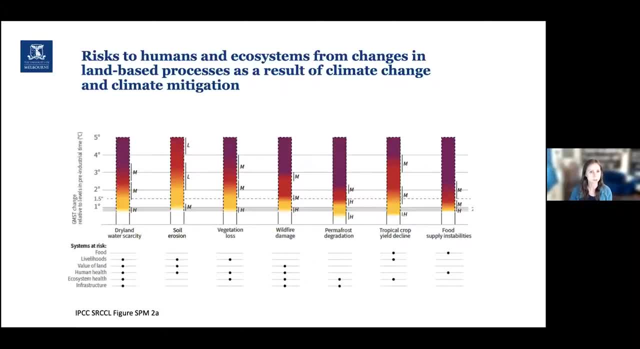 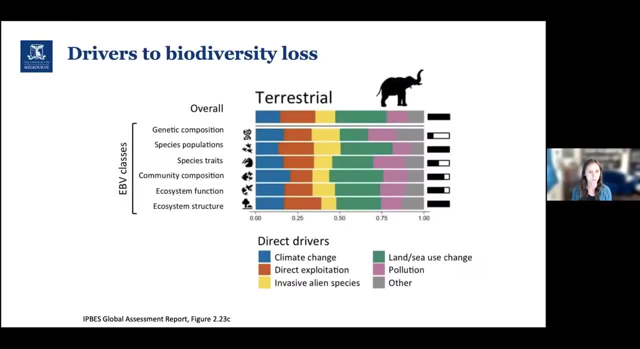 and natural systems. ecosystems result from both climate change, but also from climate change mitigation. So our response to climate change is potentially driving impacts on biodiversity and ecosystems And, in fact, when we look at what are the direct drivers to biodiversity loss, here there's 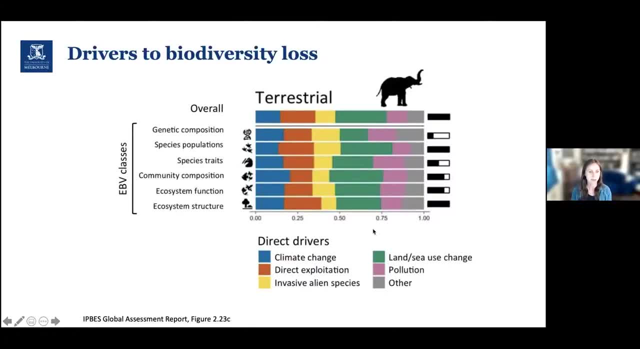 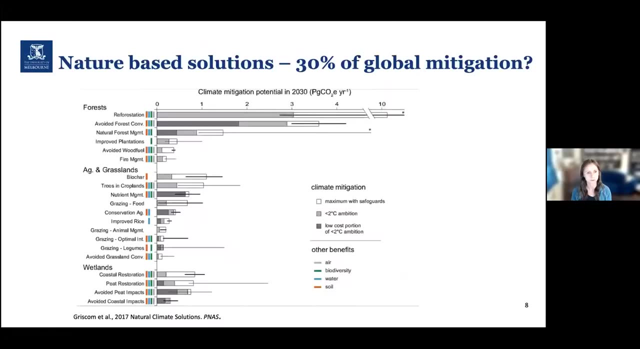 five direct drivers are characterized as five key drivers. It's actually land and sea use change is the largest. It's the leading driver of biodiversity loss. So it's no surprise that if climate mitigation scenarios rely on large areas of land use change, there'll be negative impact on biodiversity. 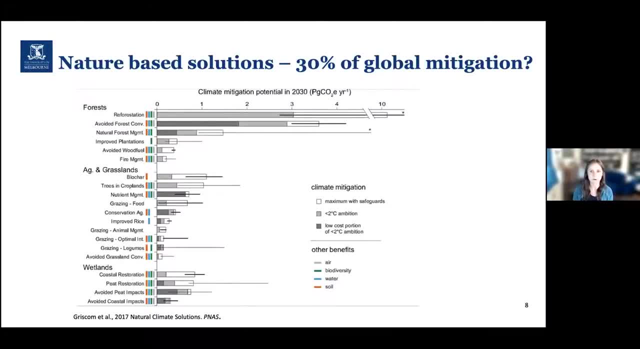 Thank you, Thank you. So this is a little bit where the whole conversation about nature-based solutions came from. The dilemma of how do we achieve that carbon dioxide removal without negative impacts on land led to this phrase, as well as a lot more focus on land-based mitigation. 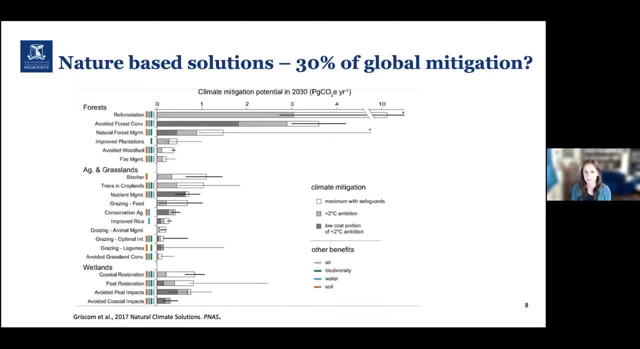 and on how ecosystems can contribute to that. Now this study is from 2017.. And it was the first study that really coined the phrase natural climate solutions And, due to quite a lot of promotion and outreach of this study, saw a huge focus on a huge pivot. 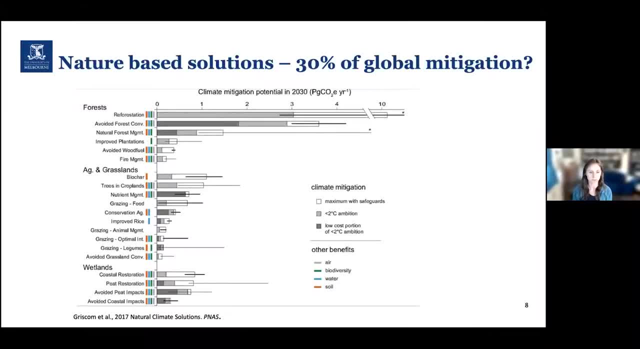 from the idea of afforestation and BECCS to achieve carbon drawdown to natural climate solutions And in fact there was a sort of a linked but slightly separate campaign- slightly linked but slightly separate- to this paper- a campaign that natural climate solutions. 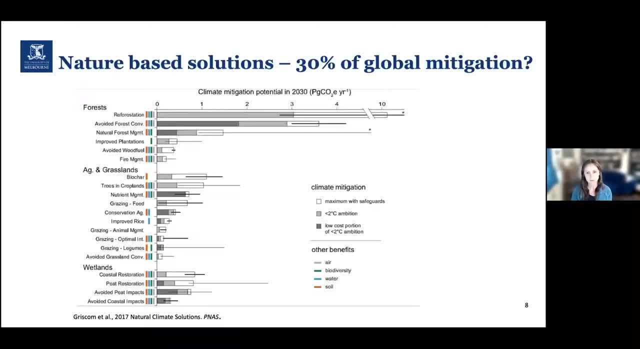 could achieve 30% of global mitigation. Now, this is really a misleading number. I think this number and the prevalence of this number in policy debates has caused quite a lot of problems. a really sort of overhyped focus on the contribution of land. 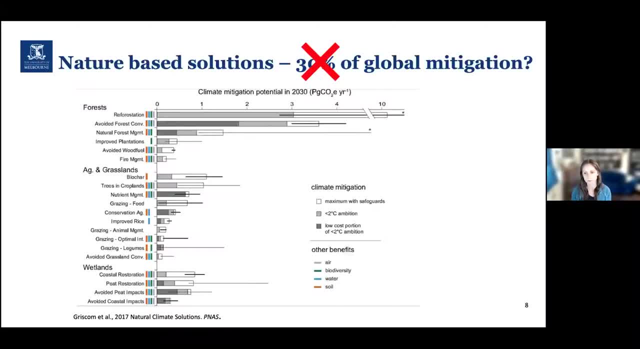 climate mitigation and has distracted from looking at what really are the range of land-based mitigation interventions that have multiple benefits and what are the limitations to land when we start in terms of its contribution to climate mitigation. So that has been a problem that is starting to be addressed. 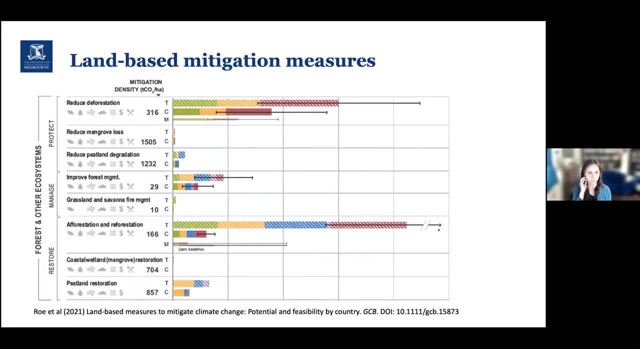 by recent papers. This is a recent study, land-based, published just a month or so ago. Stephanie wrote, and a large group of colleagues land-based measures to mitigate climate change: potential and feasibility by countries. So there's a lot of detail in this study. 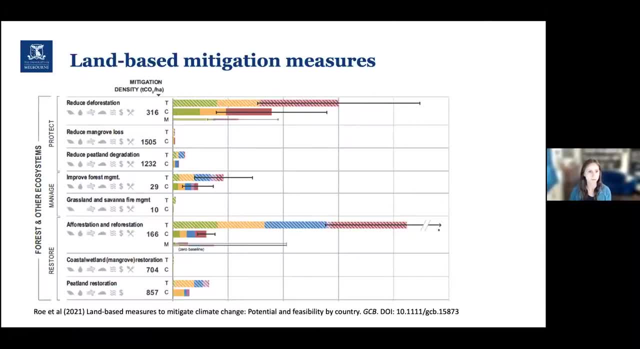 It looks at a similar set of interventions as the previous Criscum study, but it looks in more detail at a per country basis. So a lot of useful information for governments and policymakers. And they come up with a cost-effective mitigation potential of 8 to 13 gigatons of CO2. 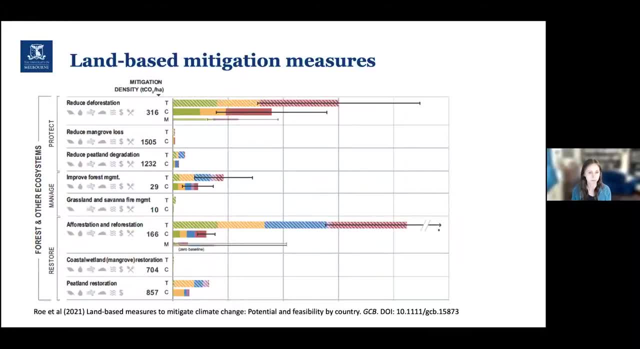 per year in the next few decades from land-based mitigation. Now this is both avoided emissions and removals, And this is a pretty. this is quite a high estimate, but it shows the potential contribution of different kinds of measures we're seeing here. 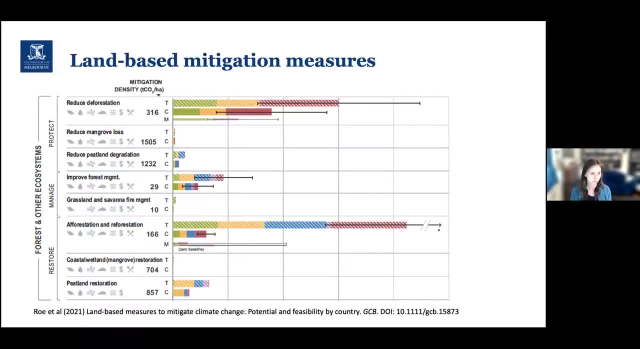 Reduced deforestation, reduced mangrove and peatland loss, afforestation and reforestation, wetland restoration, et cetera. So these are some of the options that are looked at under the heading of land-based mitigation or ecosystem restoration. 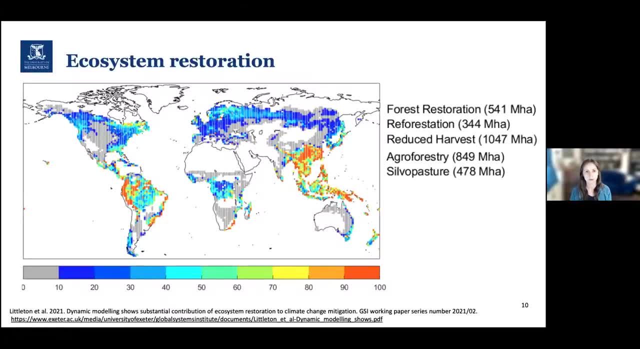 And then another- actually not a recent paper, a paper under review, but available as a preprint on Exeter University's global system institute web page. So this is a new study looking at the potential of ecosystem restoration globally to contribute to climate mitigation. 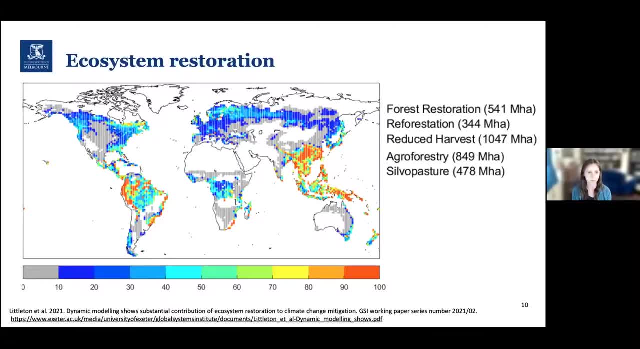 And a couple of features of this study that differ from previous ones is it very much focuses on restoration of natural but degraded forests and of degraded agricultural lands. So only looking here at five activities: forest restoration, reforestation. reduced harvest, so reduced, ongoing. 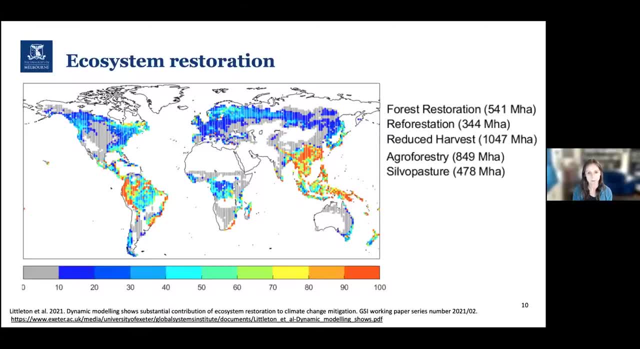 but reduced harvest in natural forests, agroforestry and silvopasture. And one of the key things about this study is it comes up with similar mitigation numbers in terms of the scale of mitigation, but much less land area And, in fact, in terms of land use change. 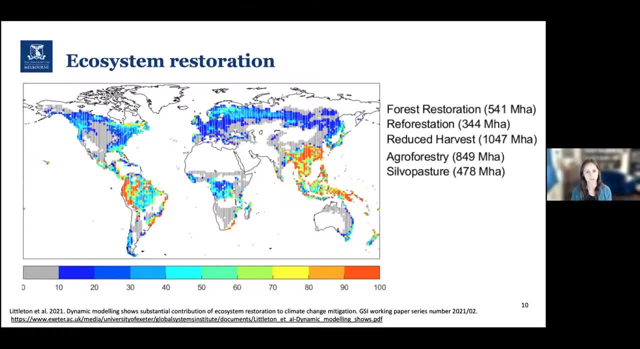 the only pathway in this study that includes any land use change is reforestation, which is an area- that which is assumed to be the area already or being pledged by countries under the Bond Challenge, So that area there is externally constrained by pledges under the Bond Challenge. 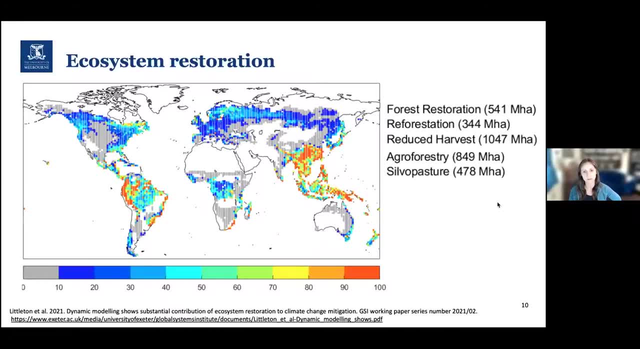 or assumed availability under that. whereas the rest of the land areas? there's no change of land use, So existing natural forests are restored. Areas that are currently used for commercial harvest continue to be used, apart from in the tropics, where research shows that there's no sustainable way. 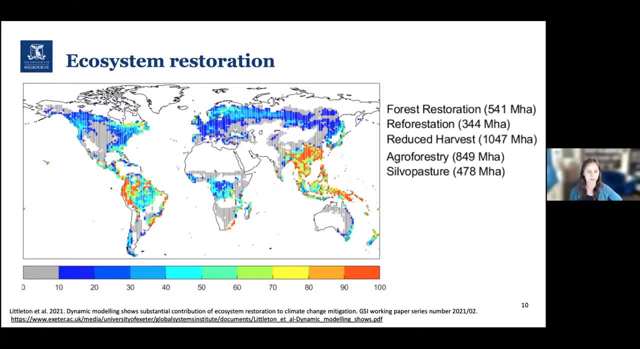 to harvest tropical forests- There's all kinds of any kind of harvest leads to decreased carbon stocks, whereas the situation is slightly different in temperate and boreal forests, And then agroforestry and silvopasture is increasing vegetation on currently farmed lands. 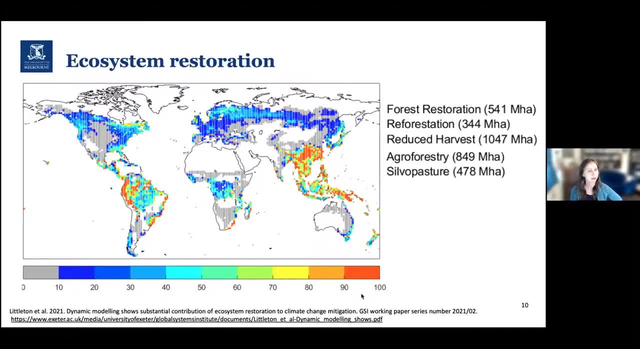 So really important. the important message here is to think about land-based mitigation without changing the land use. Can we improve existing current land uses, contributing to increased productivity on farms, increased biodiversity and ecosystem integrity in forests, and also climate mitigation, but without the negative impacts that we see. 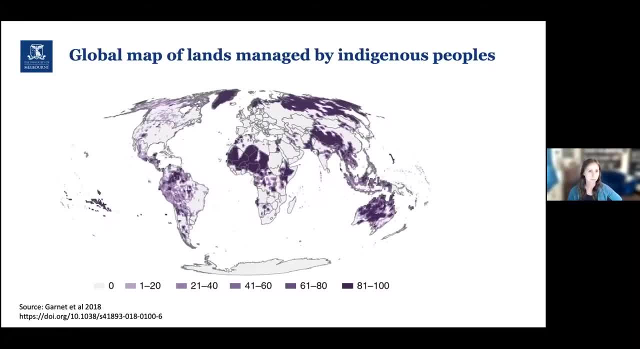 from the initial approach under the SSPs, And another feature of this new paper that I was just discussing is we consider existing land uses of Indigenous and traditional communities, such as subsistence agriculture. we consider those as necessary and part of those traditional land rights. 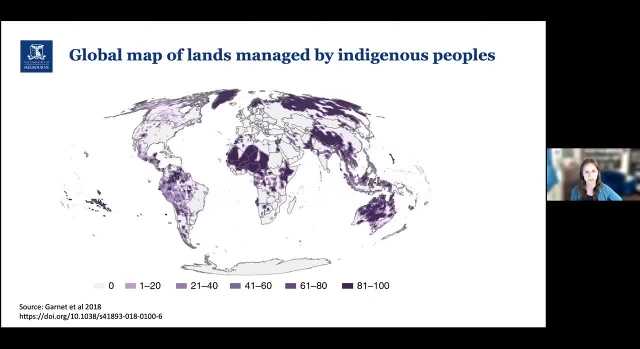 And so these are often subsistence agriculture is often targeted as a mitigation measure. There's a lot of uncertainty in how the emissions from subsistence agriculture are measured, often incorrectly measured to be very emissive activity when over longer time scales it can in fact 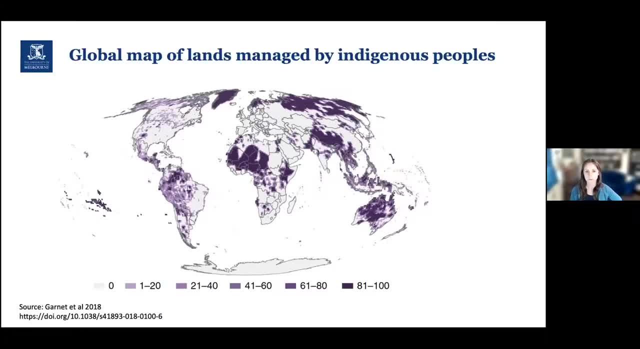 be a carbon sink of sorts. So we eliminated all of those activities from our paper And what I really wanted to emphasize here in terms of we didn't assume to reforest areas of subsistence agriculture, What I wanted to emphasize here is the 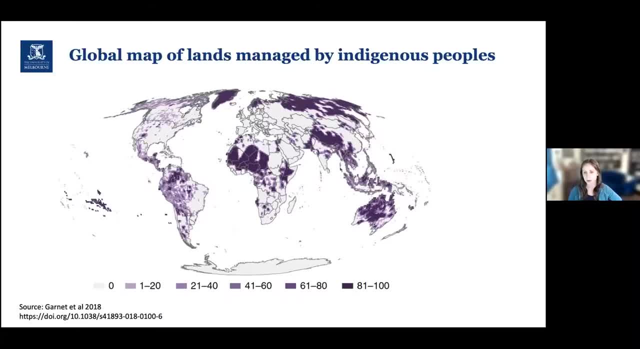 so this is a paper, also from a few years ago, that I'm showing the extent of traditionally managed or community or collectively managed land areas across the world. it best reports as being at least one quarter of the global land area. Other estimates are much higher. 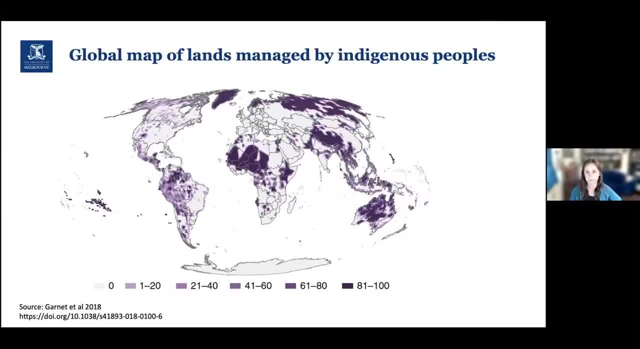 And this paper is showing that these areas of collective land management intersect with 35% of the area that formerly protected areas and 35% of all remaining terrestrial sort of intact and healthy ecosystems, And this is not a coincidence in terms of the land management. 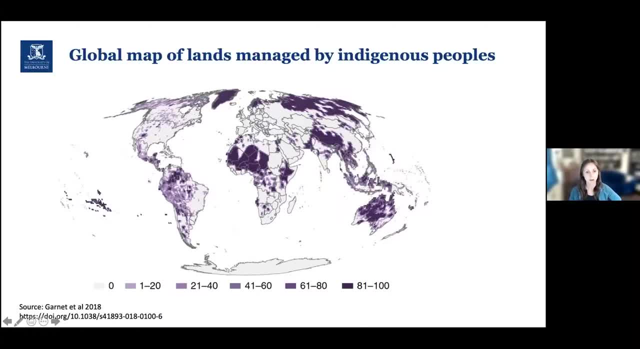 from indigenous peoples and local communities tends to foster intact and healthy ecosystems and contributes to biodiversity, climate mitigation goals, et cetera. So the importance of recognizing these land rights like community-based interventions for successful nature restoration really needs to continue to be highlighted. 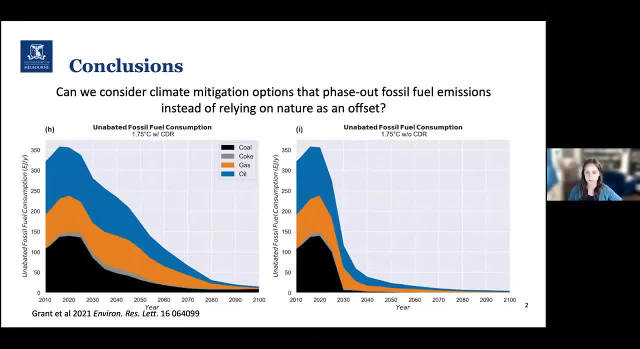 So that's kind of it from my quick overview. I hope it made sense to give some context and background And the conclusion here. the point I'm really trying to make is that nature is not. we shouldn't view it as a solution to climate change. 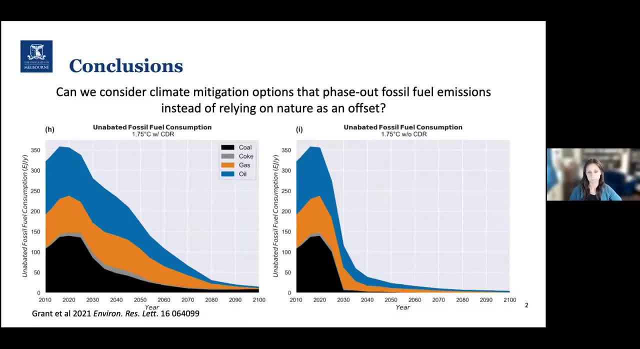 Healthy and vibrant terrestrial and ocean ecosystems underpin life on Earth, So we need to restore ecosystem integrity. We need to do this through community-based approaches, But we also need to consider climate mitigation options, potentially that phase out fossil fuel emissions instead of relying on nature as an offset. 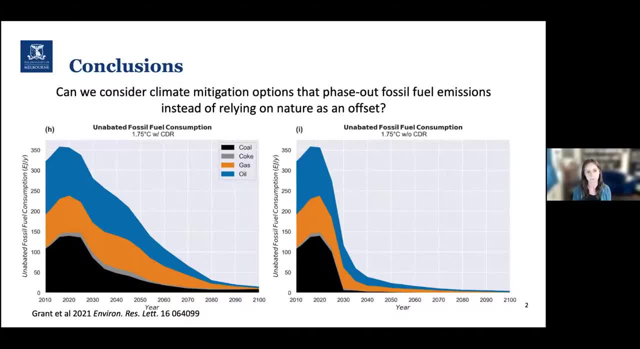 This is another paper showing the steeper reductions needed in fossil fuel emission phase out if we don't rely on nature to offset our ongoing use of fossil fuels, And I think this is part of the conversation when we talk about nature-based solutions or land-based mitigation. 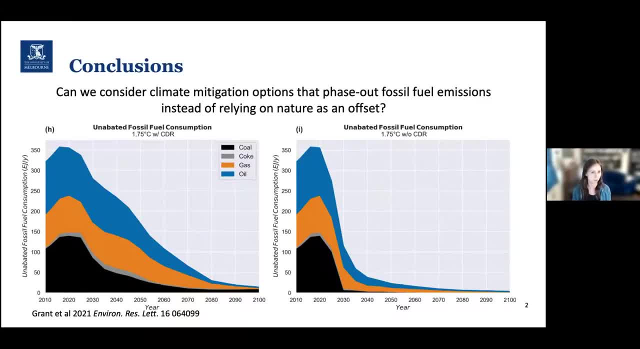 It's really important to look specifically at the policies, what's happening on the ground, the best ways to do This, which is what Kelsey and Bonnie are going to do in the next presentations, But it's also really important to keep this in mind. 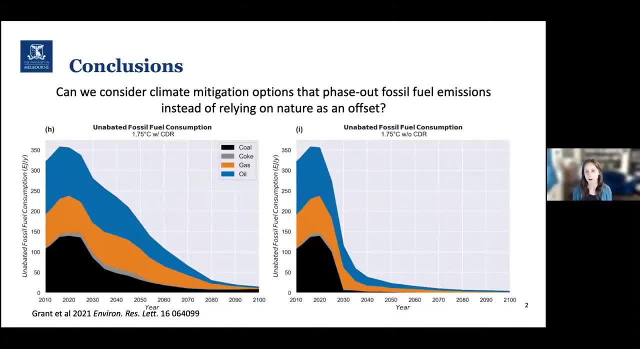 if we want to keep warming below 1.5 degrees, Offsetting ongoing fossil fuel emissions with natural climate solutions won't achieve that. And just before I finish up, actually, I realize I forgot to tell you one of the most important findings from the new paper that I highlighted. 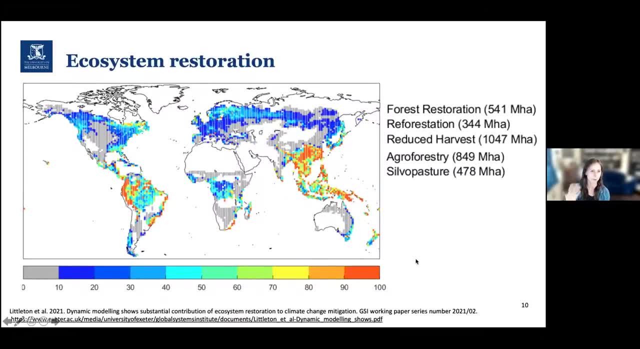 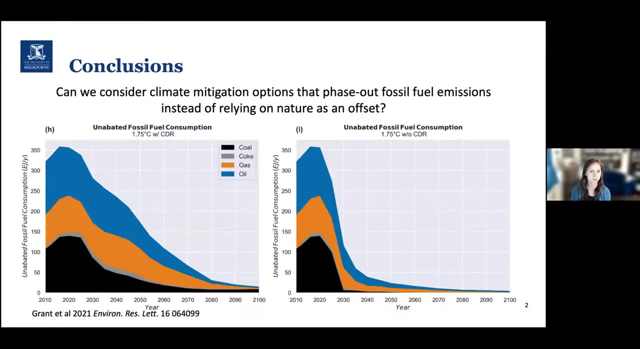 This one is that, as well as looking at how much carbon dioxide removal- carbon drawdown- could be achieved through ecosystem restoration, we looked at the impact of that on global warming, and it had no impact on reducing peak temperatures, because temperatures are going to peak in the next 10 to 20 years. 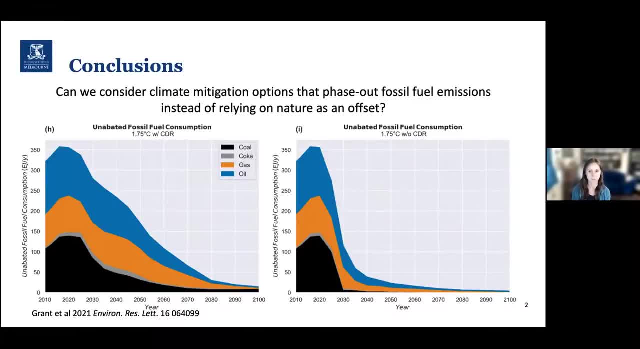 and it takes that amount of time for land-based mitigation measures to scale up, and it reduced end-of-century temperatures by approximately 0.01 degrees. So the contribution of nature, while it's really significant, and it's significant in so many aspects of human life, 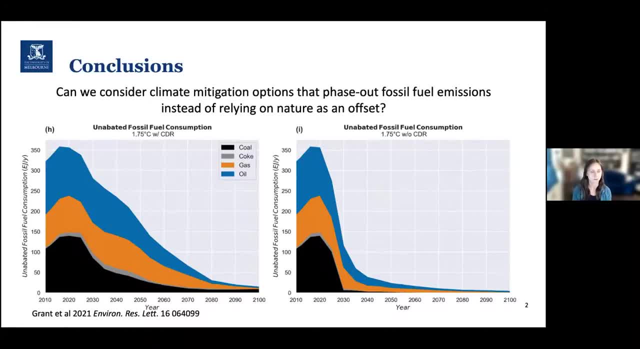 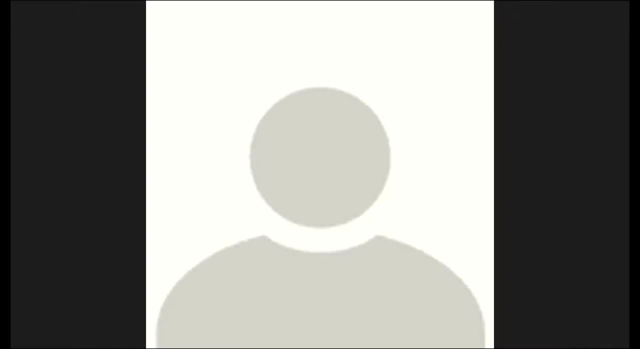 it's not. it's dwarfed by the contribution of fossil fuels to global warming. So that's hence these conclusions. OK, thank you very much. I will pass on to Kelsey next for her presentation. Great, Let me just click all the buttons. 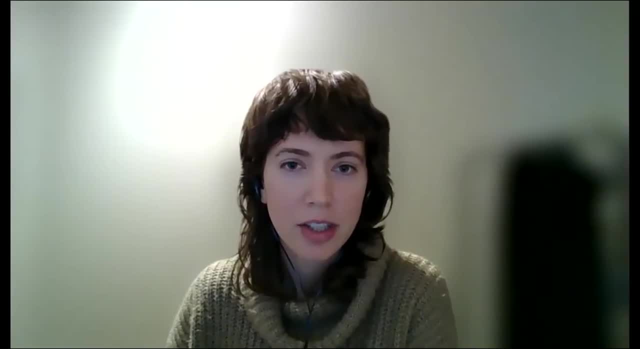 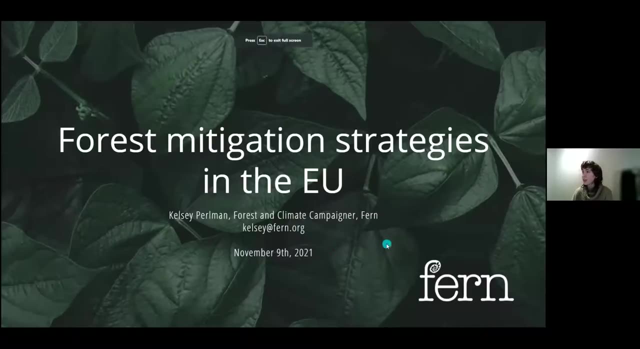 to switch on my video and share my screen. OK, great. So I'm going to be talking. well, first hello from Brussels, where I'm based, and today I'm going to be talking about some of the new mitigation strategies that the European Union has put forward. 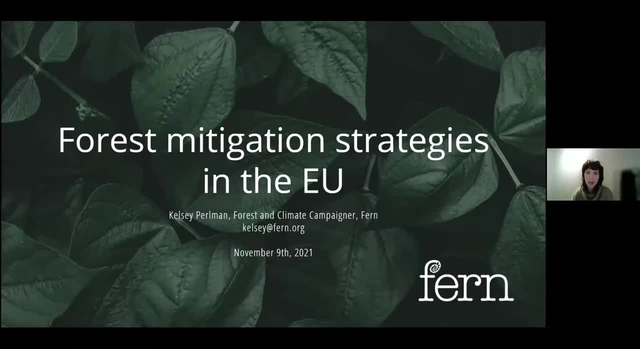 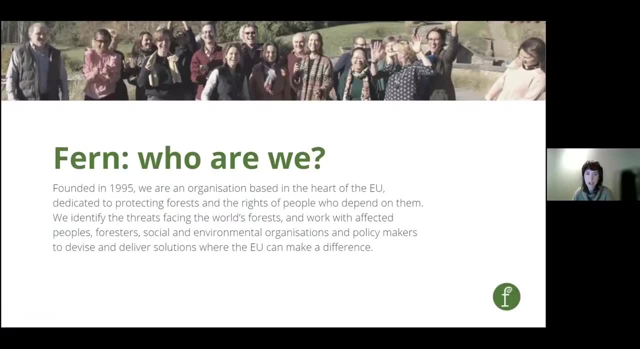 to address both biodiversity loss and climate change mitigation. For those who don't know FERN: FERN has been around for about 26 years now. We're based in Brussels and we work specifically on European Union policies that affect forests inside and outside of Europe. 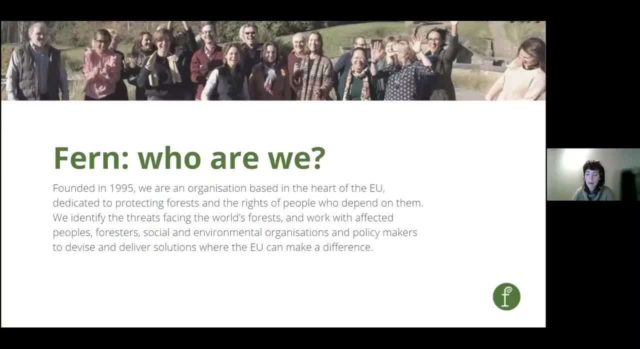 I am a policy officer working on everything related to European forests and currently we're working with academics, foresters, national civil society groups and broader EU networks on the policies that we'll be talking about today. So the OECD has been working on a number of policies. 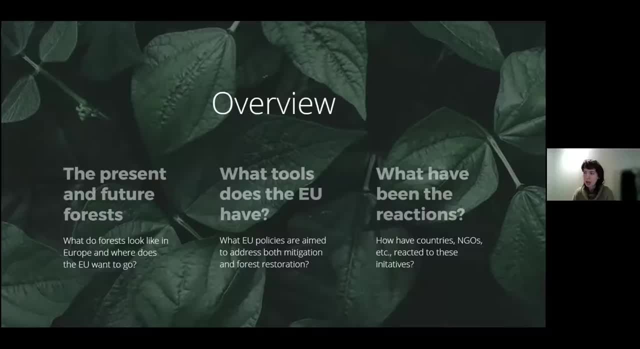 So the overview that I want to give is a bit of a snapshot of the presence, of what forests look like in the European Union and a bit the direction that the European Union wants to go, and then talk a little bit about the tools that the EU has, with a specific focus on the biodiversity. 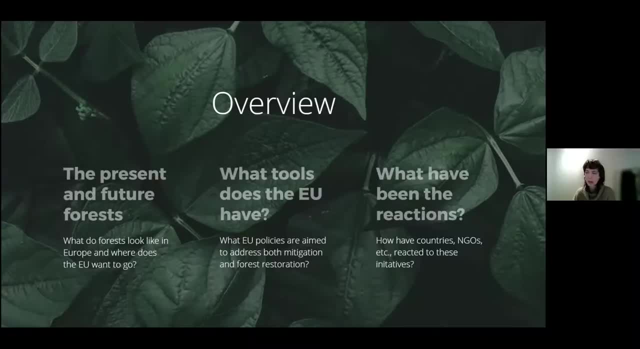 strategy and the forest strategy, which have both recently come out with a variety of initiatives that need to be interpreted a little bit to understand their impact And then look very briefly, OK, And then look briefly at sort of the reactions from NGOs, from countries, to see how these new measures have been understood. 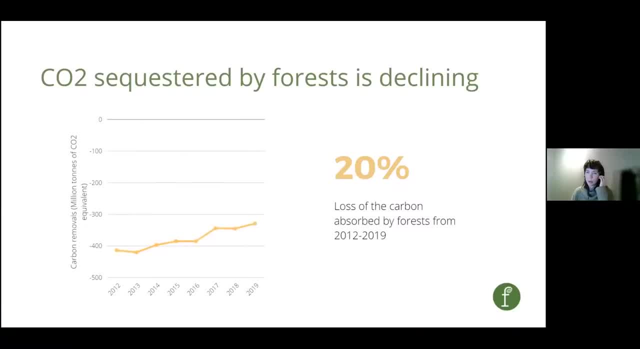 by various stakeholders. So we'll start a little bit with the mitigation angle. The CO2 that's being sequestered by forests in Europe is declining. So this information is from the European Environmental Agency. It's looking at CO2 sequestration year on year. 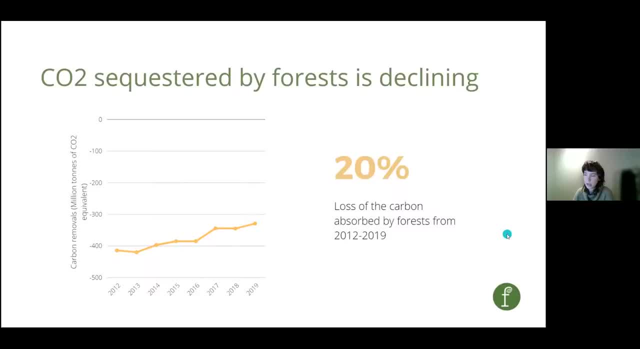 from the recent past, so this is from 2019 to 2012 to 2019, which is the most recent figures that we have. You see a 20% loss of the carbon that is absorbed by forest. I'm not going to touch on it much in this presentation. 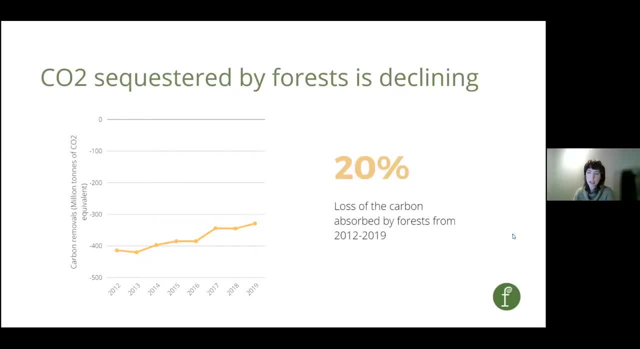 but you could argue that this is because the current land use, land use change and forestry target is actually lower. It's around a sequestration level of 225 million tons And you can argue that's one of the reasons that's drawing down. 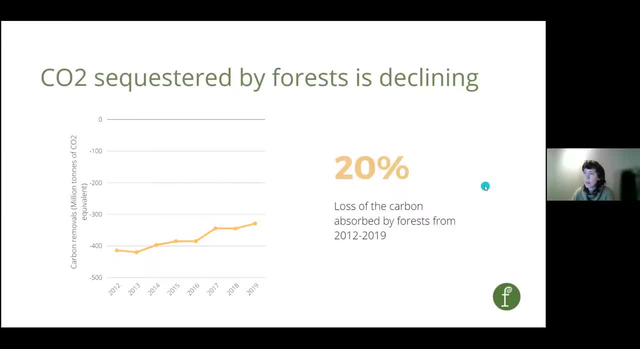 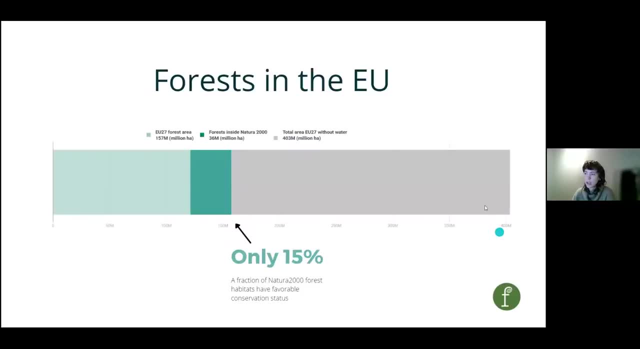 carbon sequestration So rapidly in forests. But this doesn't give a very good picture of what biodiversity looks like across European forests. So this image is basically an overview of the European Union landmass, So the area that's in gray is all other land. 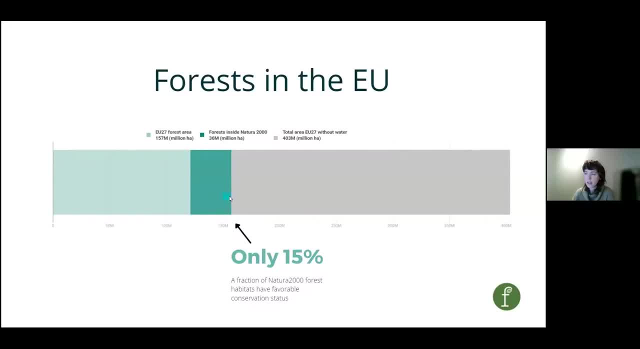 and the area that's in light teal and dark teal are the forests in the EU. Now, what's interesting about this is that the dark teal are the forests that are inside protected areas, So this is known as nature 2000 sites in Europe. 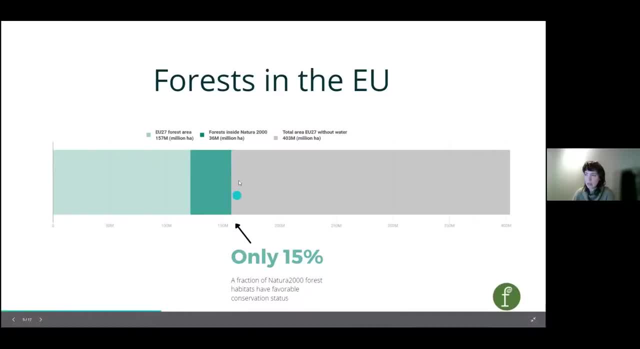 And the figure that definitely stuck out to me was that only a sliver of this, so only 15% of this smaller sliver of forests, are considered to have favorable conservation status. So it's worth noting that, in terms of monitoring for biodiversity in general, it's only this darker area. 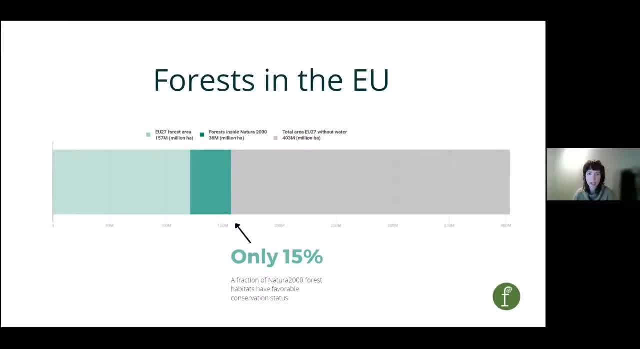 that is monitored thanks to European Union legislation, The rest of it, So the area- we have a good understanding of carbon uptake but we don't have sort of EU-wide monitoring to actually understand what's going on in all of these other forests which. 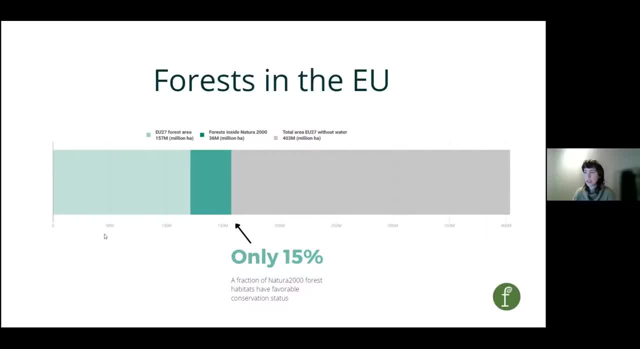 are significantly managed, And so this is something that we're going to return to, Because if we know that a very small amount of these forests that are monitored are in poor conservation status, then that begs the question of what the health of the rest of the forests across Europe look like. 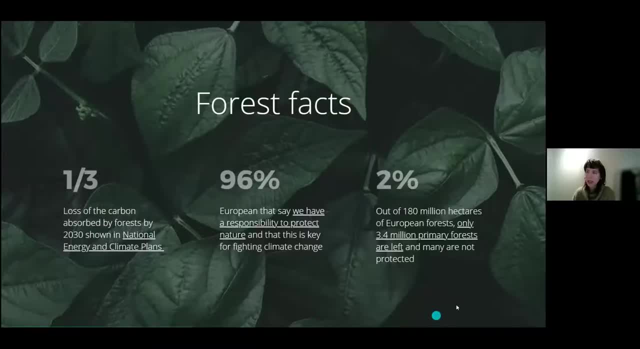 And we'll return to that question in a little bit. So some additional forest facts that may stick out. Many of the countries in the European Union have plans for the next 10 years And this degradation of the land use sink is set to continue and worsen. 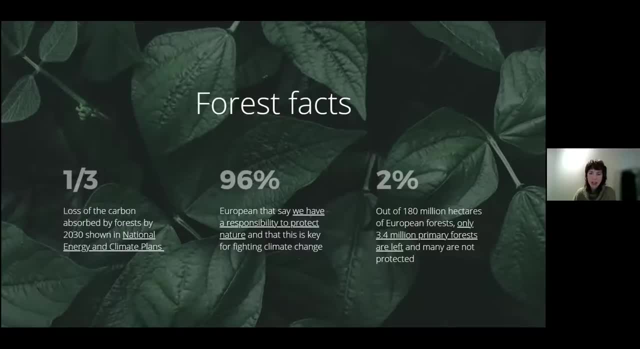 So if we look at national energy and climate plans over the next 10 years for all of the European Union member states, we're looking at a 30% drop in the loss of carbon that's stored. At the same time, we have a lot of European Union citizens that. 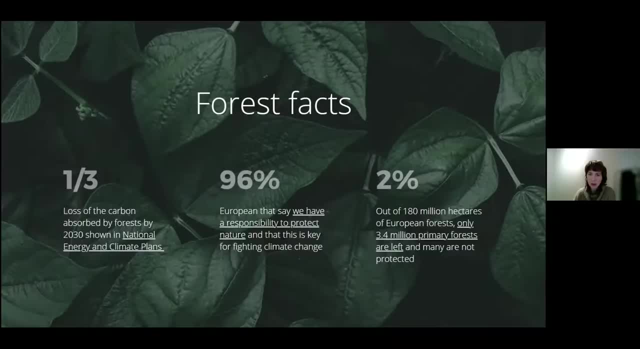 are calling For more action to protect nature and come forward with legislation, which is what the European Union is planning to do as a sort of a key action to address climate change and biodiversity loss. And then, finally, if we zoom in on the primary forest, 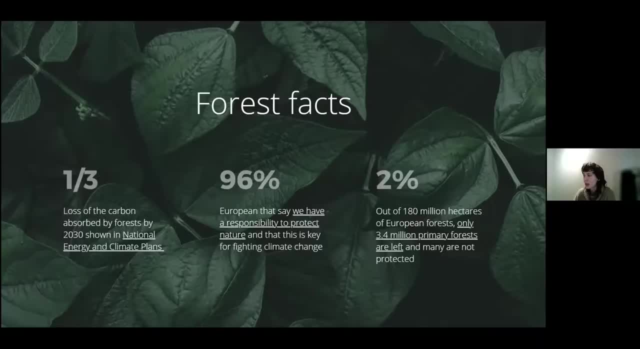 we don't have very many left in Europe, But we have about 3.4 million hectares, And many of these do not find themselves in the protected areas, which was quite surprising for me. So there's still some action to be done in that area. 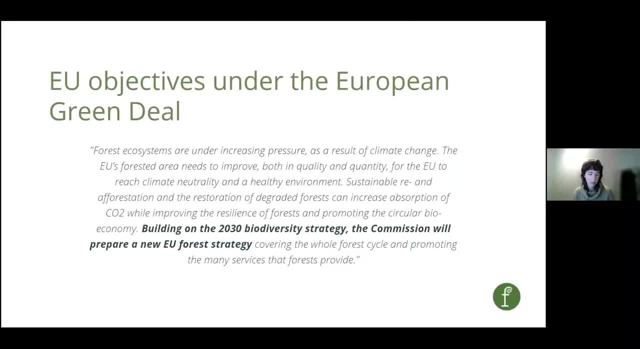 So, as kind of a context setting before we discuss the biodiversity strategy and the forest strategy, sometimes it's difficult to understand how these two strategies interrelate with one another. This comes from EU objectives that have been put forward underneath the European Green Deal. 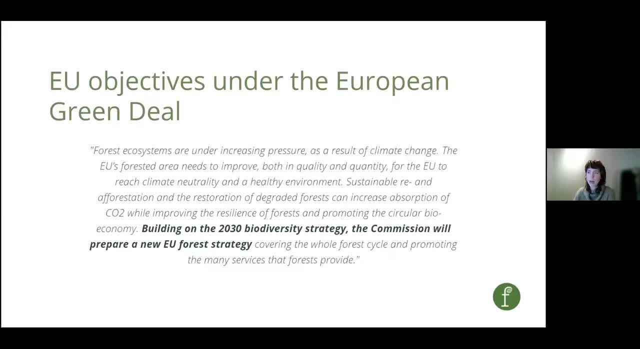 So this is the paragraph- one of a few paragraphs that are on forests, because the Green Deal covers all sectors And it lays out very clearly that it's basically building on the biodiversity strategy, which has set out some headline objectives. There will be a new forest strategy that's 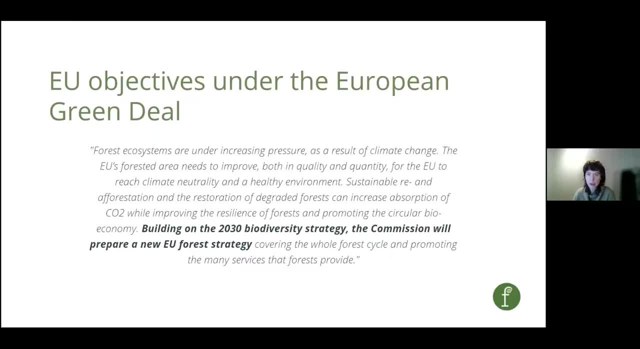 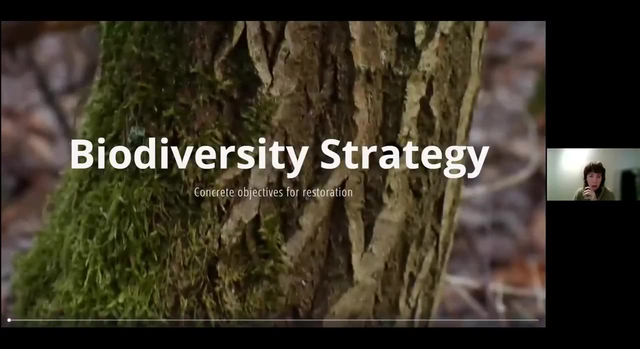 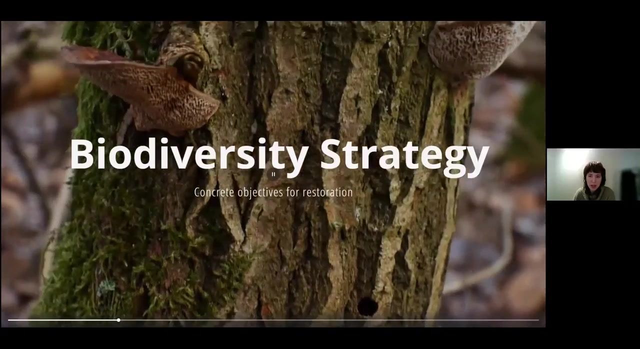 produced to attempt to cover the entire forest cycle and have a more holistic approach to transforming forest management practices and biodiversity protection. So now we'll take a look at the biodiversity strategy. This has very specific Objectives for restoration and we'll look at those a little bit more in depth. 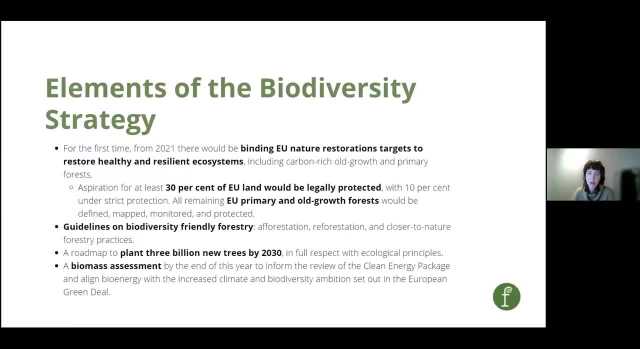 So, for the first time in 2021, there's going to be binding EU nature restoration targets. Now, what separates this from the last strategy is that there were voluntary targets that didn't have timelines set And those voluntary targets were not achieved. 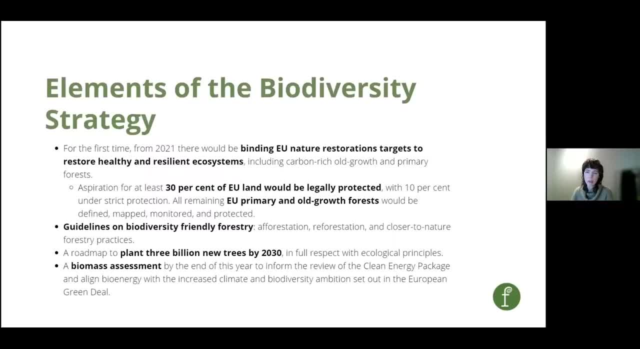 So the change this time around is to come forward with a law that's going to put out a target for how much needs to be restored And basically detail out definitions and require a bit more in terms of what needs to be done. So this is the headline action. that's. 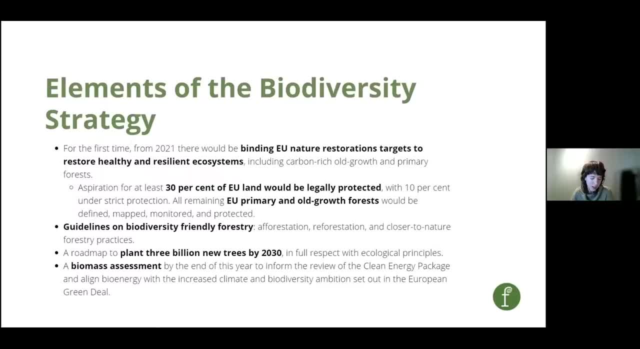 underneath the strategy. Any strategy can consist of laws, which are the most binding thing that can come forward from such a document, aspirational goals, roadmaps for projects where you hope to have buy-in from many of the countries, And you can also have reports and things. 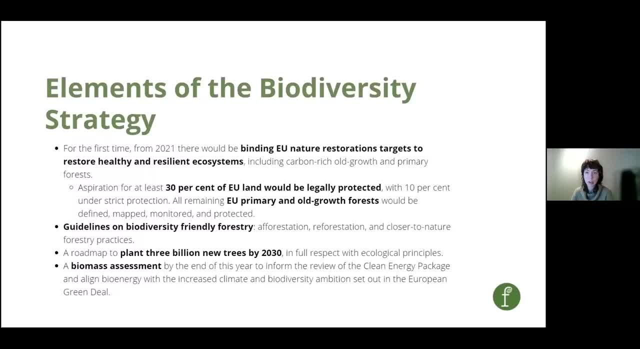 like that. So, of all of the things that you see in this document, it's really the law that most people are responding to when they comment on the ambition of the strategy. So, in relation to that, you have an aspiration for a wider coverage of the Natura 2000 areas, which 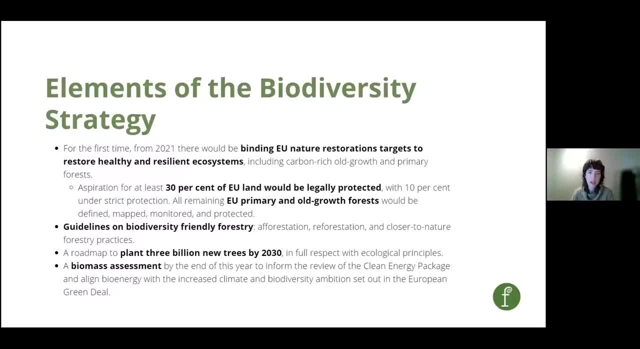 you saw on the bar in a previous slide- to cover at least 30% of the EU land. Right now it's around 23%, with a certain amount of that underneath, And you can see that the EU has a very strict protection. 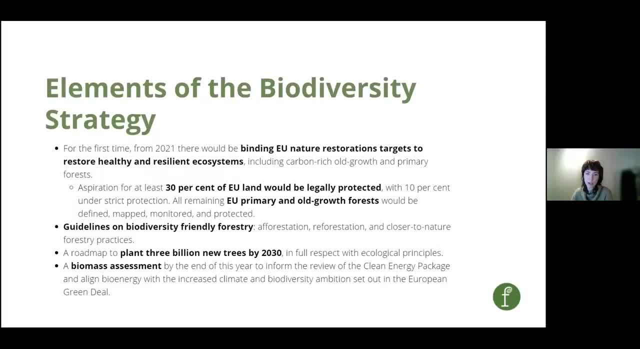 Part of this is to define and map primary and old growth forests in the European Union to be able to facilitate the protection of those, And you'll see that the definition slightly changes between certain member states. At the same time, you have guidelines on biodiversity-friendly forestry. 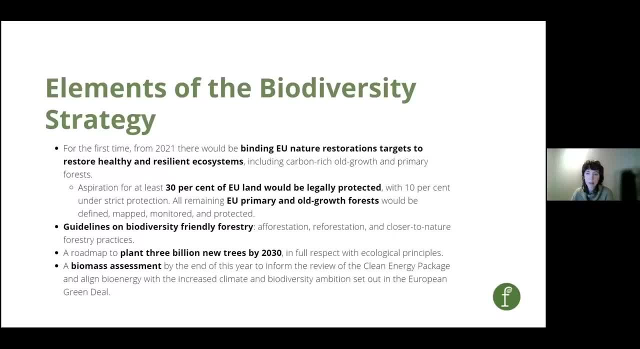 So there are three different sets of guidelines that are being developed And this is a bit of a technical exercise that can potentially feed into other initiatives. It can feed into the nature restoration discussion as well. So there are guidelines on biodiversity-friendly afforestation and reforestation as one area. 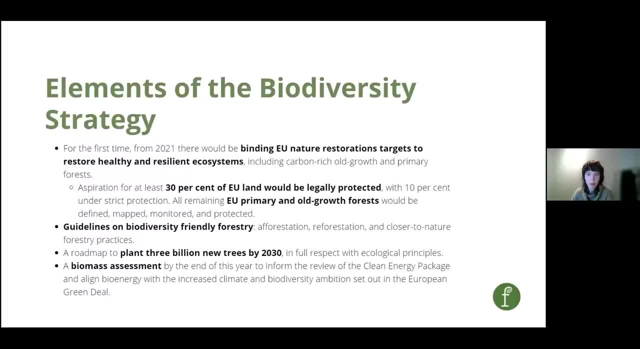 There's the work on old growth forest, which is also a set of guidelines, And then there are guidelines on closer-to-nature forestry practices, which is an effort to further define forest management criteria to be able to more effectively and more accurately determine what the impact of management. 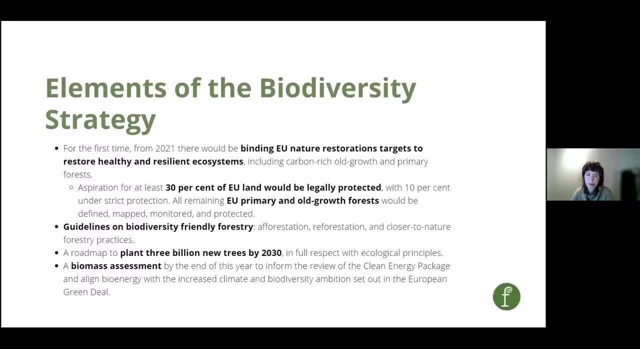 practices are. Many of you may have also heard that there's a roadmap to plant 3 billion trees, So we're waiting for more information on what that will look like and what the obligations will be, understanding that this is a voluntary initiative, that's. 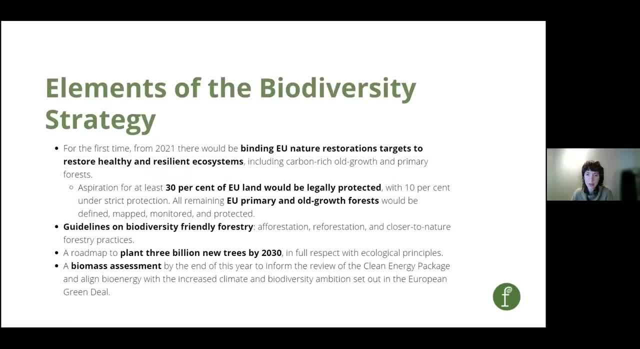 coming forward that has a lot of hype behind it, So there are a lot of questions as to what this will look like and if it will actually materialize into anything. And then, finally, they've committed to a biomass assessment to basically look at the impact of wood products on biodiversity. 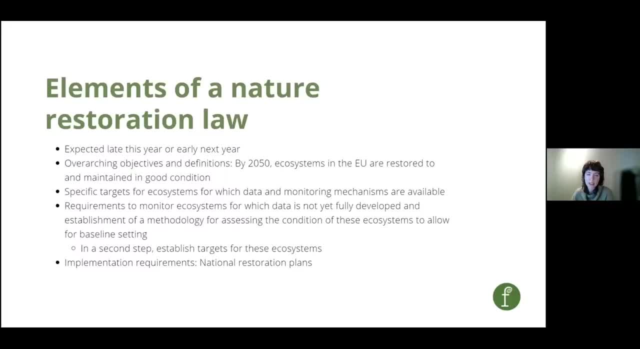 and on climate mitigation. So, as I mentioned, the strongest element of the biodiversity strategy is the nature restoration law. It's expected late this year or early next year And there are quite a lot of novel elements, So one is looking at sort of overarching objectives. 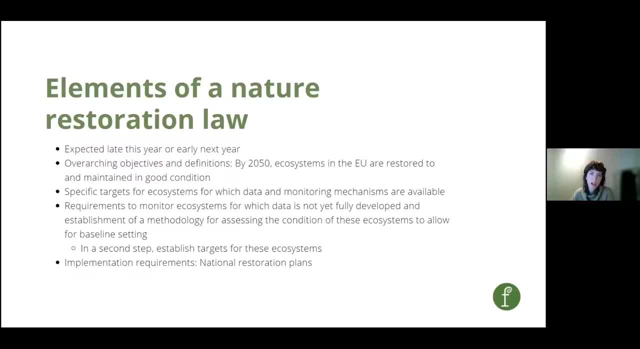 and definitions. what's been proposed so far is that by 2030, ecosystems are restored to and maintained in good condition. So there's a question about what does good condition mean? What does restoration mean? All of these things will need to be debated. There's going to be sort of a two-step process for defining targets. There's 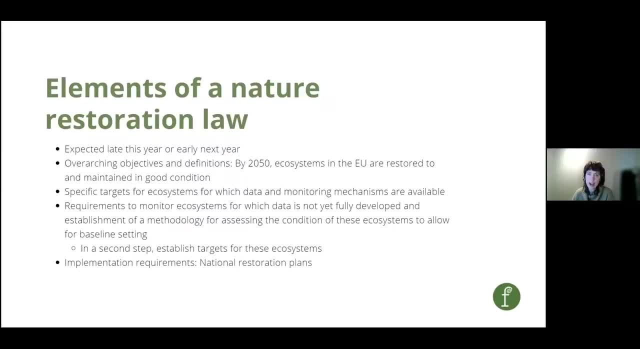 going to be specific targets for ecosystems that have data and monitoring mechanisms that are already in place. At the same time, there's going to be requirements to monitor ecosystems where there isn't sufficient data, with the goal to eventually develop a methodology for assessing the ecosystem condition of those forests and to eventually, in a second step, create targets for. 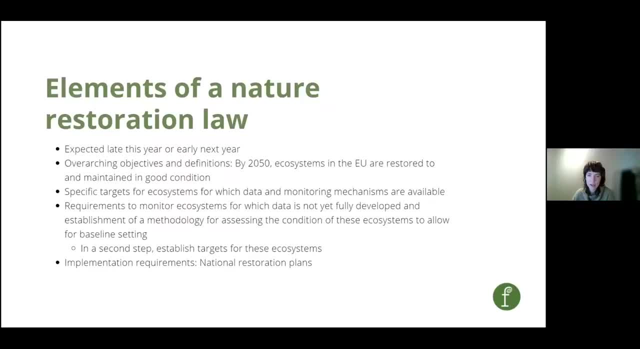 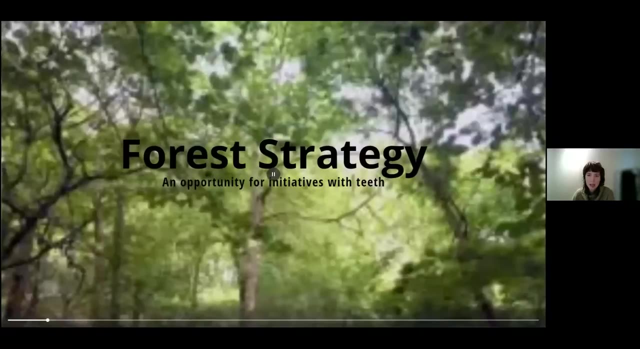 other ecosystems. And then there will also be the development of other tools to sort of help achieve these objectives, like national restoration plans. So now we can look a little bit at the forest strategy. It should be noted that Fern was actually quite critical about the forest strategy the first time around, because there 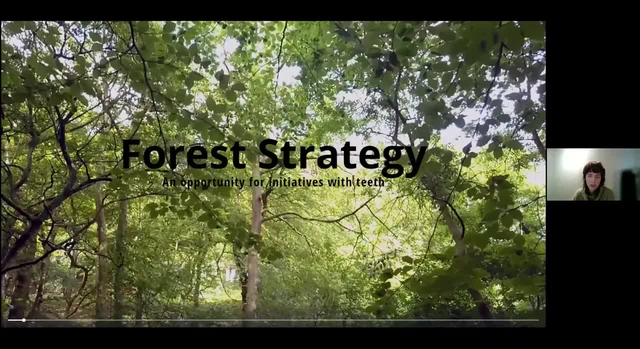 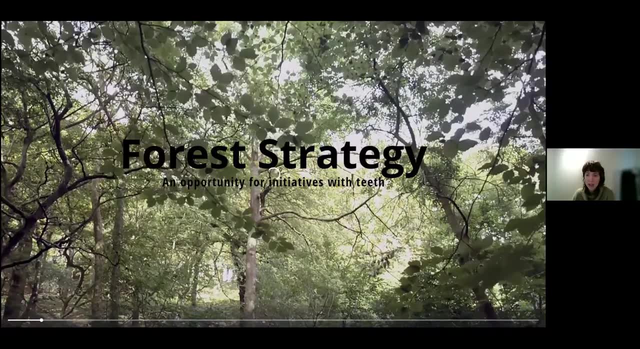 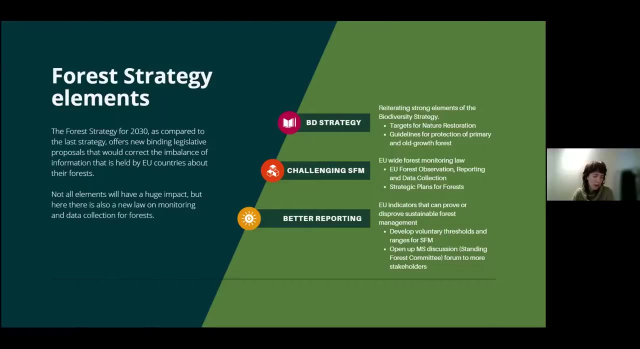 weren't a lot of binding initiatives that were underneath this strategy. This time around there's the possibility of having a couple of initiatives that have some teeth, that can actually change things, And they're sort of the technical version of a more detailed next step. 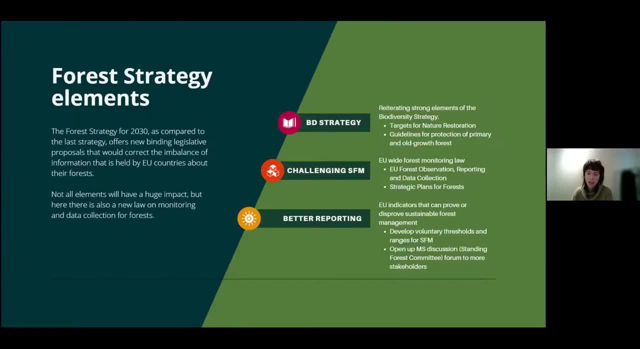 for forests that can eventually help achieve some of the objectives of the biodiversity strategy. So this is an overview of some of the elements of the forest strategy. There's basically a first element that reiterates a lot of the different initiatives that are inside of the biodiversity strategy. So it reiterates the fact that there are targets for nature restoration. 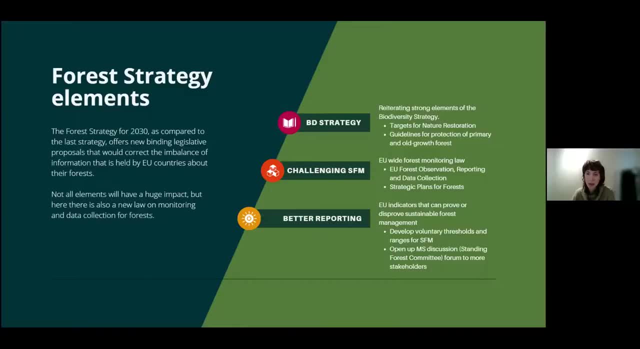 It reiterates the guidelines for the protection of primary and old growth forests. But the novel element of this and the strongest new element- so laws are the strongest, as I mentioned- is they're going to put forward in the EU wide forest monitoring laws. So this has a long and cumbersome 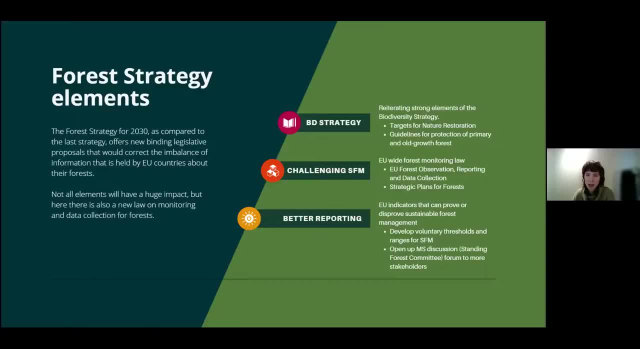 name. It's the EU forest observation, reporting and data collection law to be accompanied with strategic plans for forests over the next 10, 20 years, And so this would attempt to bridge that gap and to compile additional information to be able to strongly say what's happening- happening in the vast majorio. 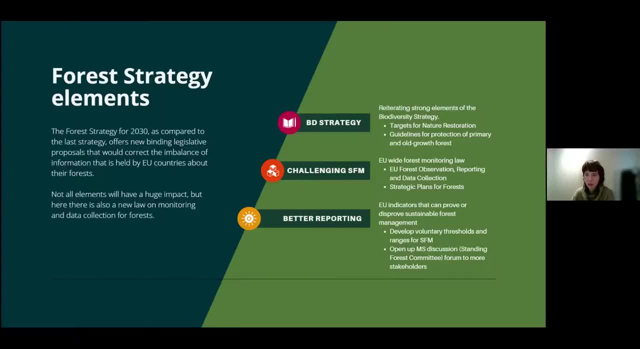 ity of the forest, forests that aren't currently covered by monitoring. So to do that, there's also the requirement of developing additional indicators for forest management, The goal of this being able to prove or disprove whether forest management is actually sustainable in the 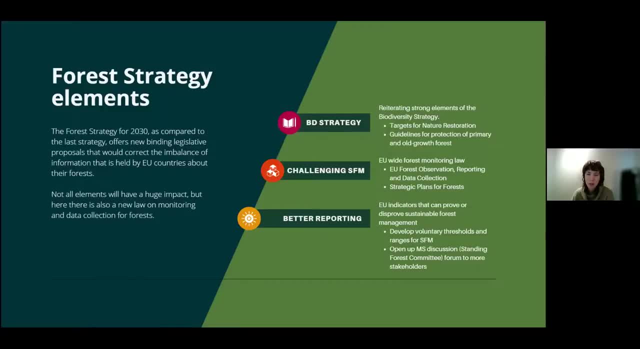 European Union. So there's been some pretty provocative comments by European Commission officials, basically saying what many of us have known for a long time: that we cannot prove sustainable forest management in Europe the way that it stands now because we don't have the indicators. We only have the red flags coming from the reporting of protected areas in Europe. 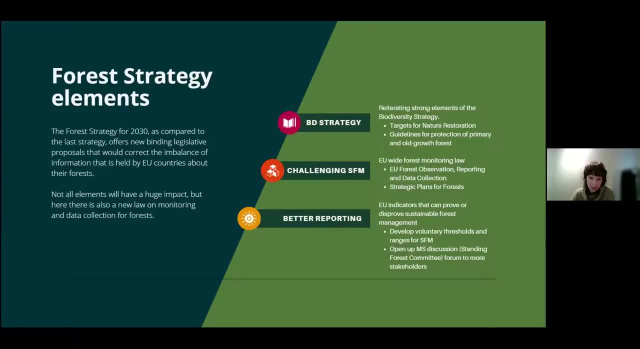 So there's going to be, as I said, the development of sort of thresholds along with these indicators. If we say deadwood is a specific indicator, then determining how much in certain biomes will be a conversation. And then, in addition to all of this, there's going to be a discussion about 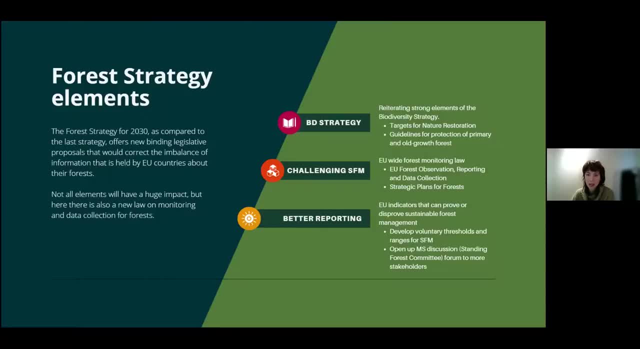 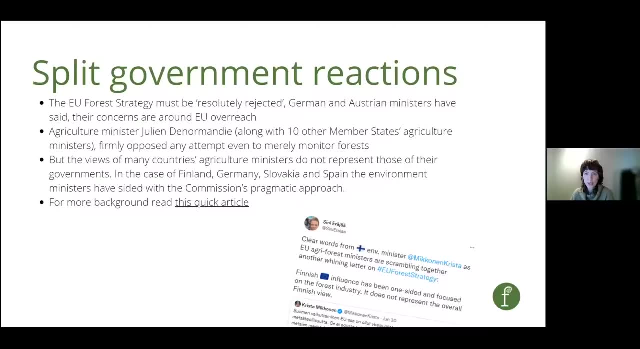 the importance of sustainable forest management in Europe. So there's going to be a discussion about how stakeholders come together to be able to discuss a lot of these issues. So, looking specifically at some of the reactions to what is essentially a request for further monitoring of forests and a conversation to be able to progress a little bit on the IHE targets, 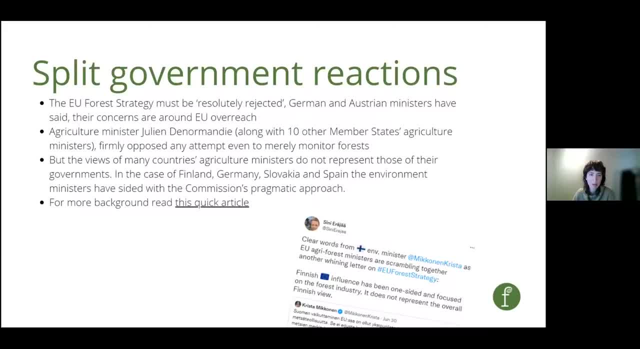 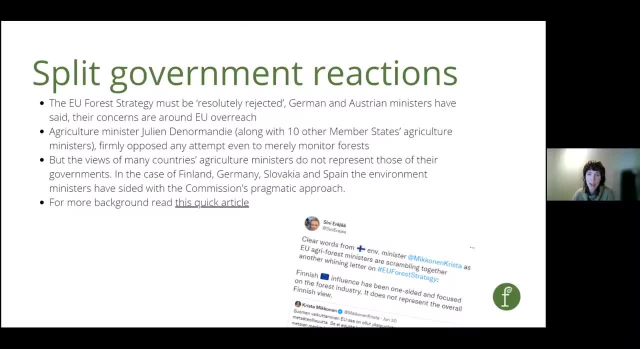 level negotiation, particularly between the management group. we need to have those kind of discussions, and so we're expecting to see pressure on this IE government from some governments. There was a letter that came out support of all of the initiatives underneath the forest strategy and the biodiversity strategy. 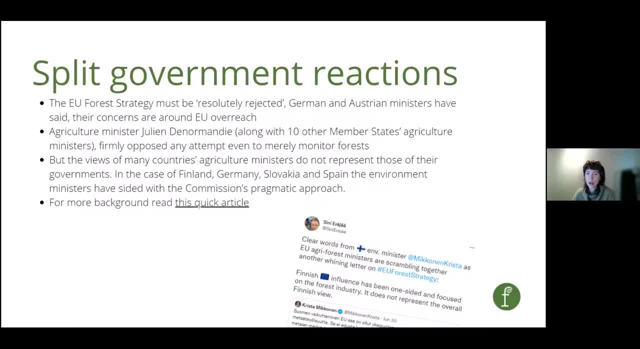 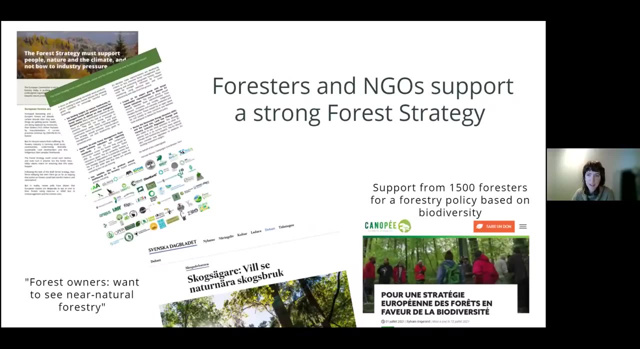 I'm sure the slides may be shared afterwards, so there's a short article basically looking at the tension between some of the agricultural ministers and the forestry ministers about these two different initiatives, but particularly about the EU forest strategy. At the same time, obviously, NGOs have come forward with a strong statement in support. 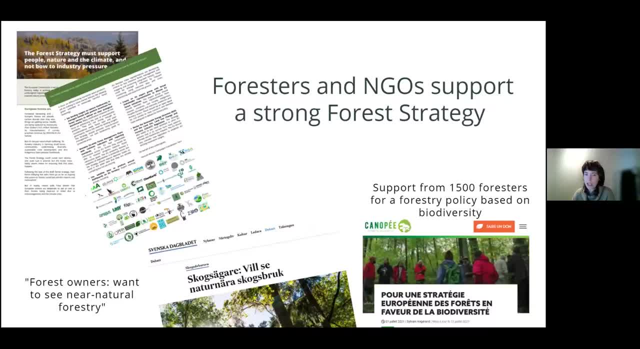 of the forest strategy. but what is more interesting in my mind- because it's a new actor that's jumping on the scene- is that there is a mobilization of foresters that are in support of forest policy that's based on biodiversity and sustainability over the 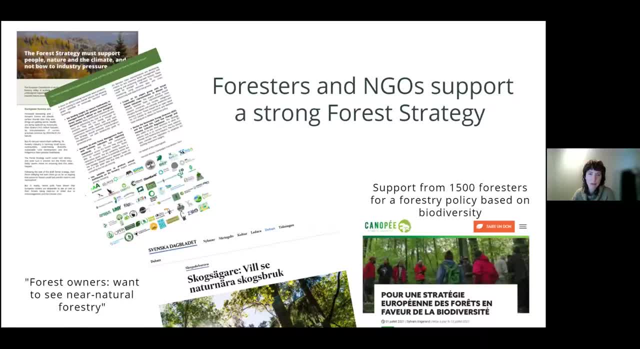 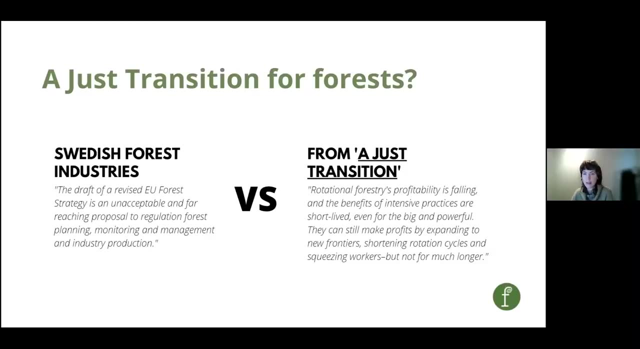 long term. So you can see a coalition of foresters from both Sweden and a large coalition of foresters from France coming together in support of basically defining what the forest strategy is, Defining what good practice looks like. So there's a very interesting conversation about a just transition for forest at the 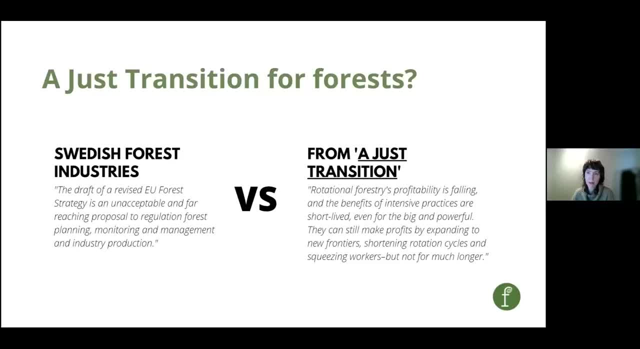 EU level We have the difference of opinion from some of the larger forestry industries versus some of the more progressive foresters that basically have very different opinions on the subject of what the future of forestry looks like. So to sort of close and recap on the opportunities, 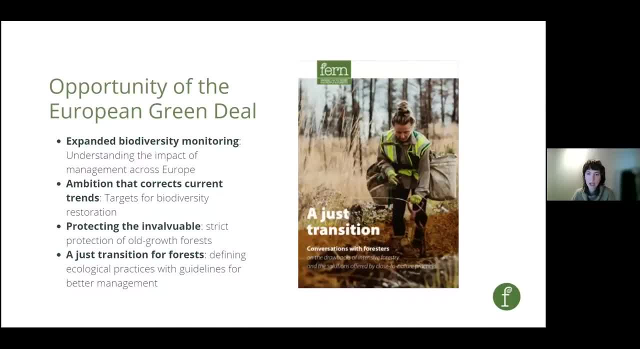 that are presented by these two files. it really is about a transformative solution to look at forestry across the EU. There's this opportunity of expanded biodiversity monitoring with the explicit goal of looking at the impact of management across Europe. There are binding new targets that will increase ambition around biodiversity restoration. 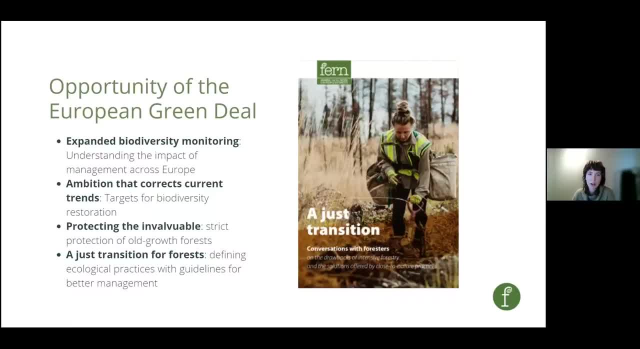 particularly, There is explicit protection for old growth forests- the few that are remaining- And there is a long term discussion that will continue over the next couple of years around defining ecological practices and defining guidelines for better management to be able to help with this land use change shift in a positive direction. 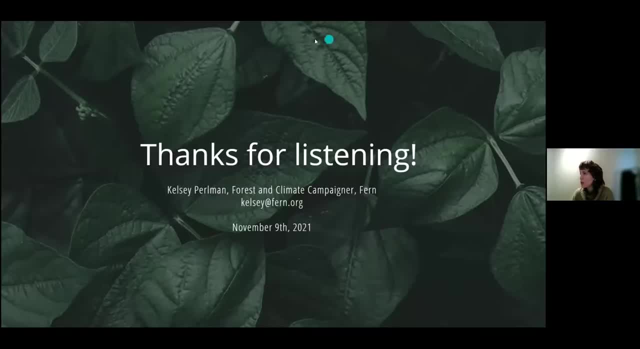 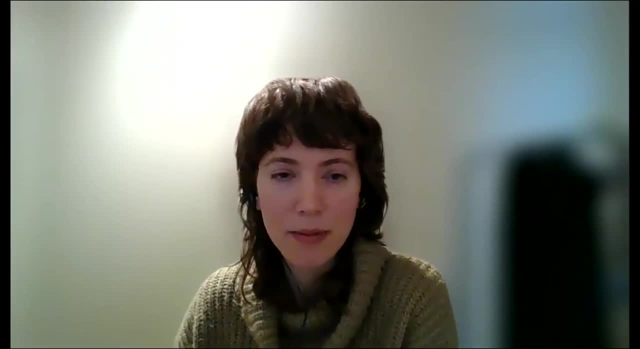 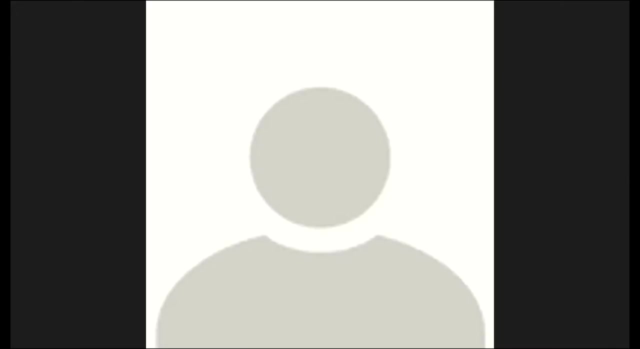 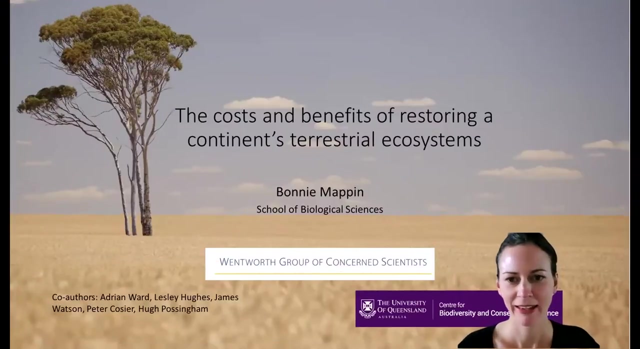 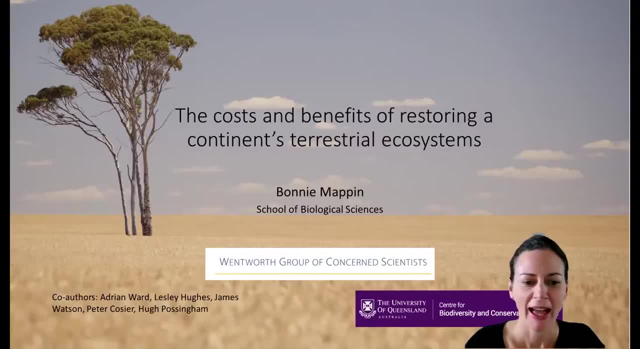 of restoring a continent's terrestrial ecosystem, And this is a really critical moment in the world And I think we need to understand that. And this is some research that I led as part of my PhD at the University of Queensland, and it was in collaboration. 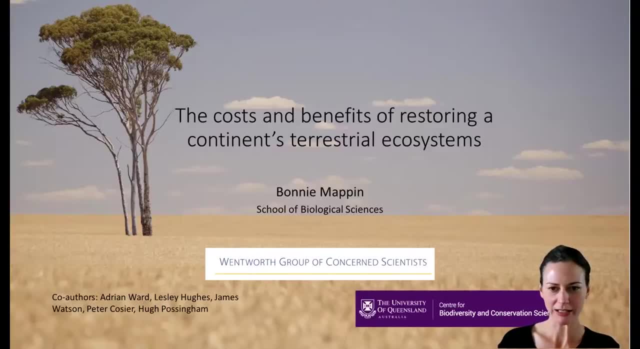 with the Wentworth Group of Concerned Scientists. The Wentworth Group of Concerned Scientists are some eminent Australian scientists that work together to gather scientific information to advocate for good, sound environmental policy. So this research is quite forward-looking and looking at the opportunities that is possible in Australia. 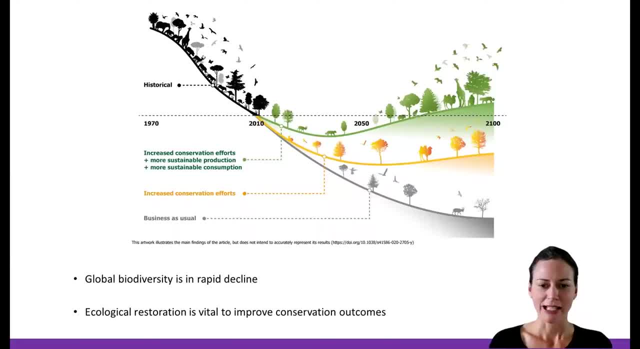 As we've touched on, humanity's expanding demands for resources is really driving global biodiversity loss and it's in rapid decline. We've cleared significant areas of land and it's being increasingly recognised that land landscape scale restoration is vital for conservation of biodiversity. 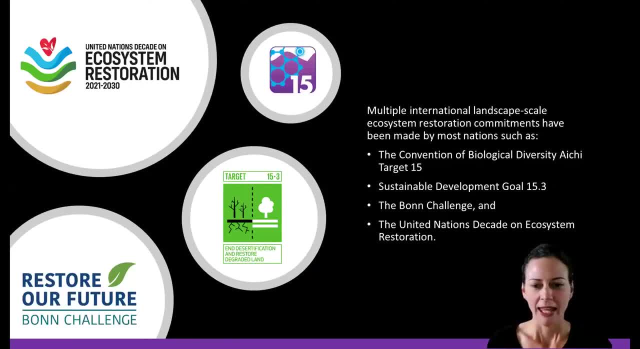 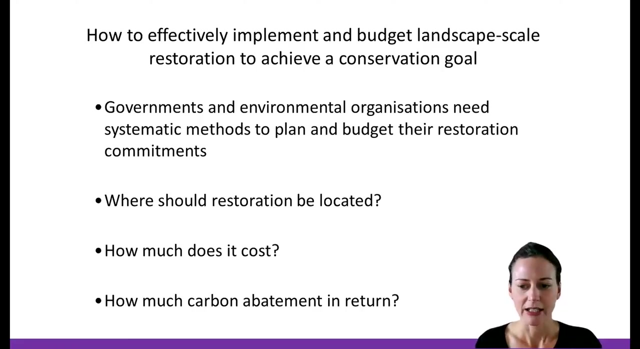 And in recent years there's also been an upsurge in grand restoration endeavours with very high aspirations for both conservation and climate change, as well as sustainable development, And these restoration initiatives do offer some opportunities to lessen anthropogenic environmental change. However, for these schemes to be effective, systematic methods are really needed to help. 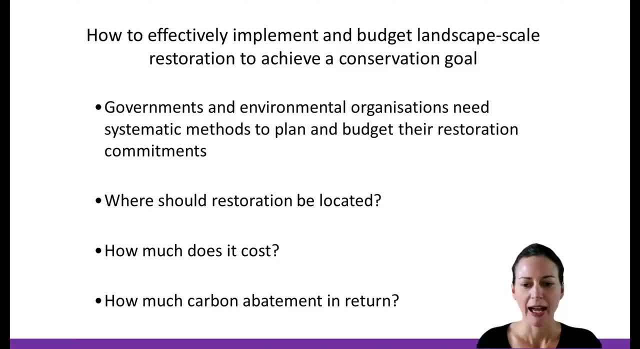 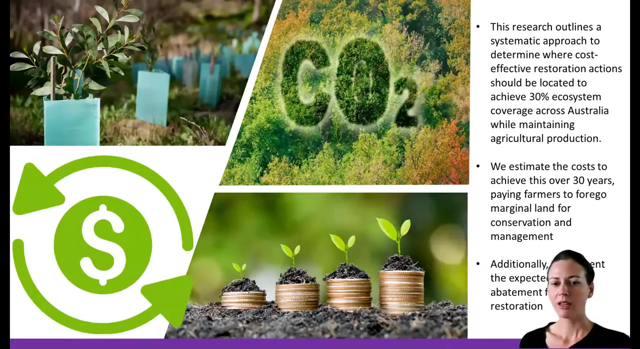 plan and budget these restoration commitments and to be able to answer questions such as: where should we be restoring, how much will it cost, and what sort of carbon abatement do we expect. So this research focused on where can cost effective restoration action be located to. 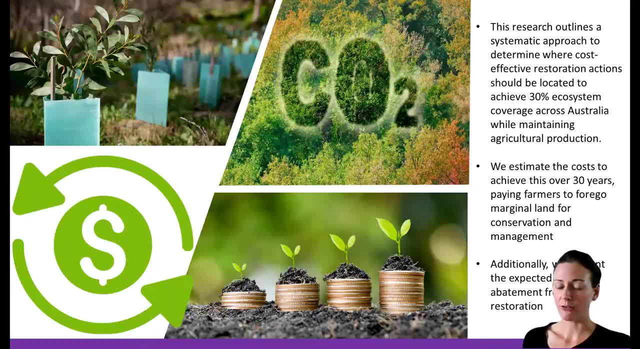 achieve a 30% coverage of all ecosystems in Australia, while maintaining our agricultural production- And we estimated the cost to achieve this over a 30 year period- paying farmers to forgo marginal land for conservation and management. We additionally present the expected carbon abatement for this restoration. 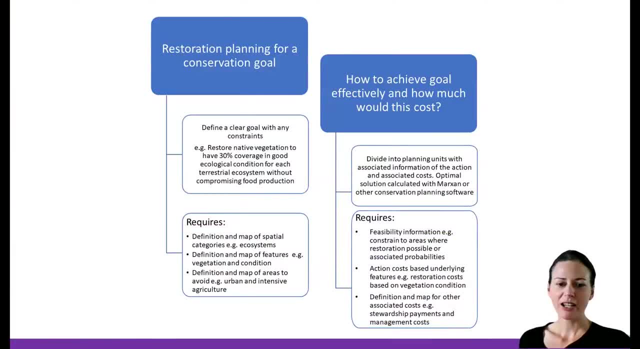 So the underlying approach that we used in this study could be applied to many other restoration projects. 1. goal needs to be defined, including definitions and gathering of spatial information to determine where restoration actions need to occur and constraints within the goal should direct the restoration efforts to locations that need restoration and bind the restoration. 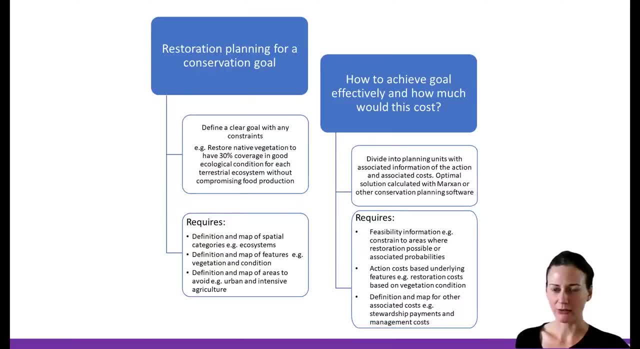 intervention types to ones that will be effective within the social as well as the ecological context, and to effectively achieve direct restoration. sorry, to achieve a conservation goal, we really need to look at the feasibility of restoration and the spatial costs that would be needed. In this case, we estimated the direct actions of the restoration costs. to do this, we 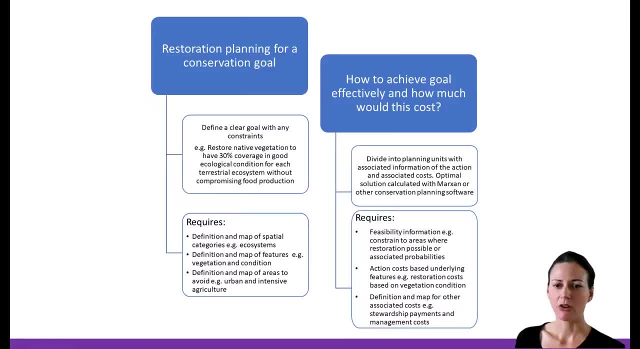 stratified the landscape based on spatial information and the spatial information that is being challenging to deal with. We also Ning talked abouit the actual perspective and the spatial context of the project that I think we would benefit from At the end of the date. you have several questions foruttoin the next two works. 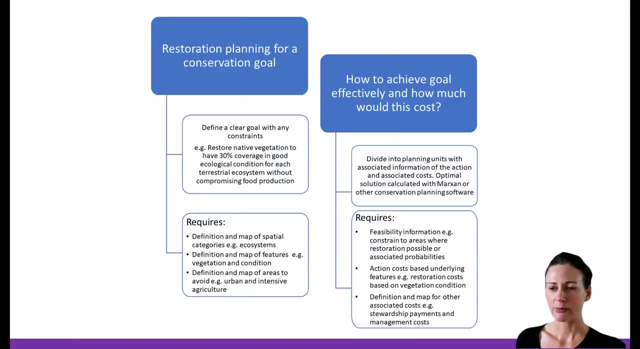 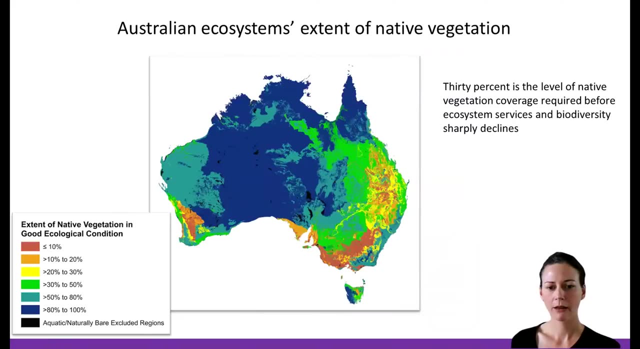 In this project we worked on the information on vegetation as well as the situation, and we excluded areas with low restoration potential. so in our case, urban, industrial and intensive agricultural areas, And this sort of framework could be adapted to be updated with more accurate information and a different conservation goal. So in this research we firstly defined the 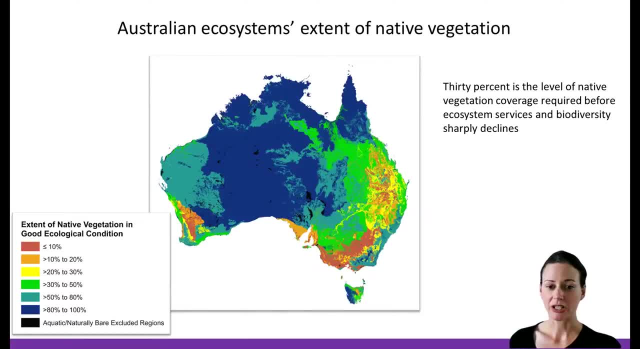 current extent of native vegetation in a healthy condition in Australia across all our ecosystems. Now we identified which ecosystems have less than 30% coverage and why this 30% number is key is that it is a threshold in which, below that point, ecosystem services and biodiversity have. 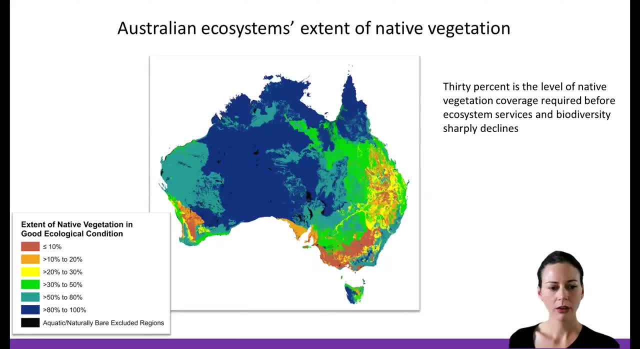 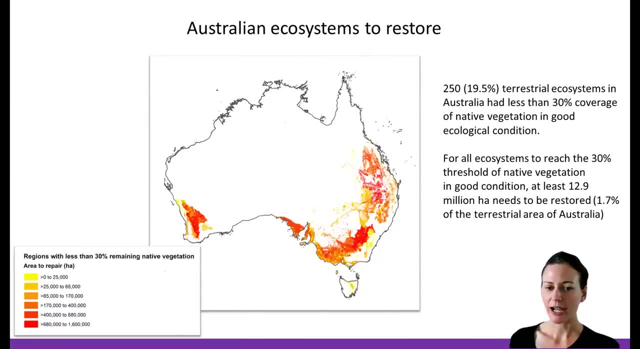 been shown to sharply decline, and so we found that 250 of our ecosystems have actually got less than 30% coverage of native vegetation, and to be able to reach this threshold of 30% of all ecosystems, we would need to restore 13 million hectares across Australia. This is about 1.7% of area of Australia. 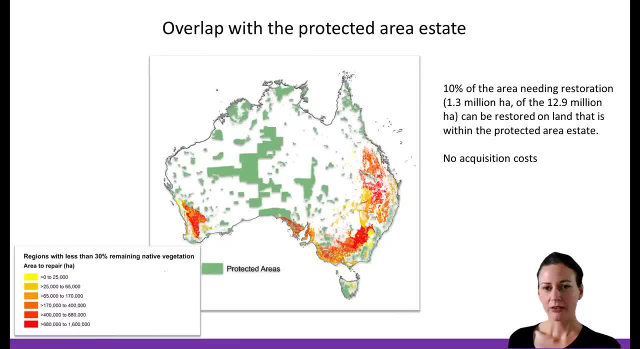 To be cost effective. we first looked at finding solutions within the current protected area of state. so these are areas that are already dedicated to conservation, wouldn't require any further acquisition costs, and we found that there is actually 10% overlap of area needing restoration that are already in these established conservation areas. 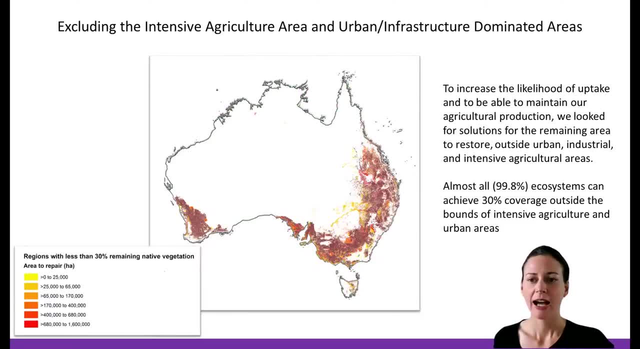 Next, we looked to exclude the areas of urban, industrial and primary agricultural areas which, as you can see, highly overlap with these areas that have been heavily cleared. However, we actually find that 99.8% of all ecosystems can actually reach this 30% level outside these areas. 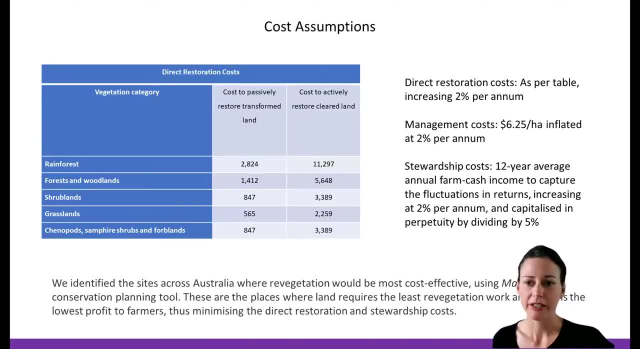 To estimate the cost to restore these areas, we included three types of costs: Direct restoration costs, stewardship costs and management costs. In the case of the direct restoration costs, we base this on both the vegetation type as well as its degraded condition For the stewardship. 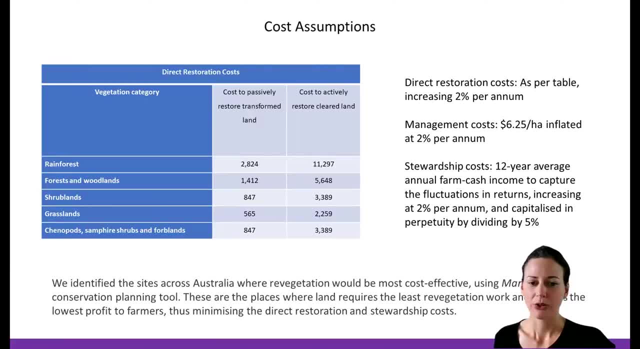 payments. we base this on farm income, so profits that farmers were seeing on this land, and we capitalised this into perpetuity, so compensating farmers to forego this land. We would see this rolling out in an opt-in scenario where farmers can choose to diversify their income, to retire some of their land and be compensated for it. 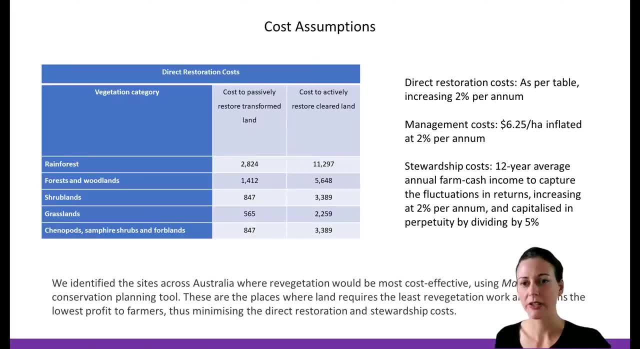 For the management costs, we left this as a flat fee across the landscapes or a cost per hectare, And this was based on averages of existing programs in Australia. Then we identified which would be the most cost-effective sites to achieve the 30% target across Australia. 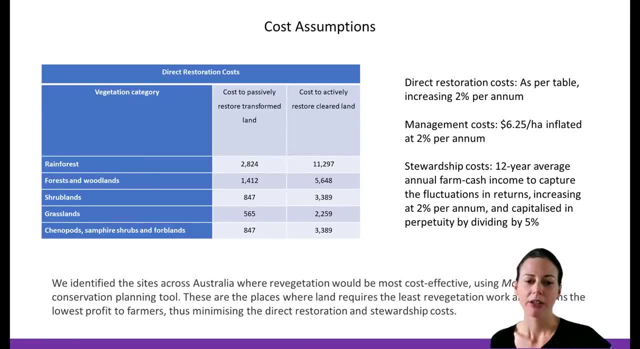 And we did this by minimizing the direct restoration costs as well as the stewardship costs. Sorry, my head's in the way, but basically that would be using. I used a tool called MarkSan, which is a conservation planning tool that we can break down that information to small spatial scales. 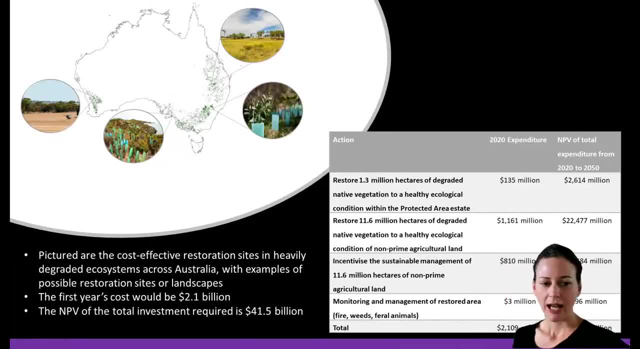 And here I present the results. So pictured is the most cost-effective restoration sites, And these are examples of possible restorations, And here I present the cost information. So we estimate that if this was done over a 30-year time period, that the first year it would cost about $2.1 billion. 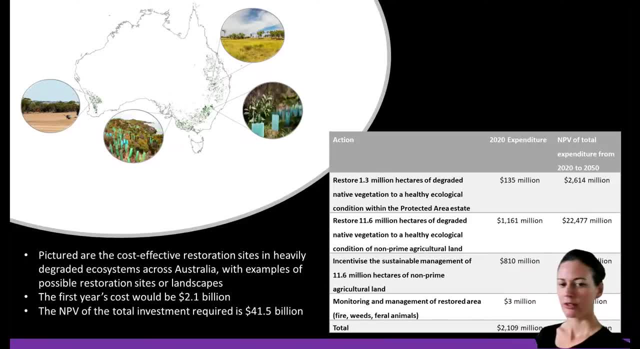 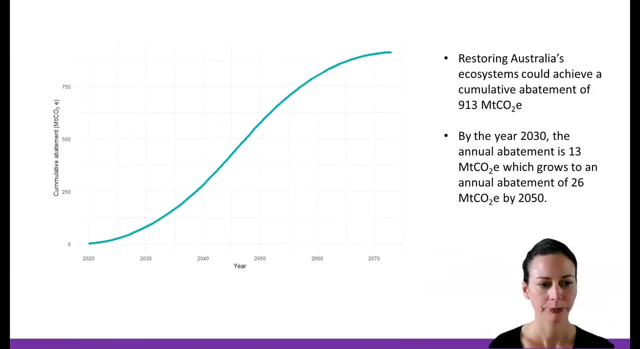 And then the net present value of the total investment over the lifetime of the project would be $41.4 billion. Now the carbon benefits would flow in over not only just the 30 years of replanting but the 25 years post that as trees mature. 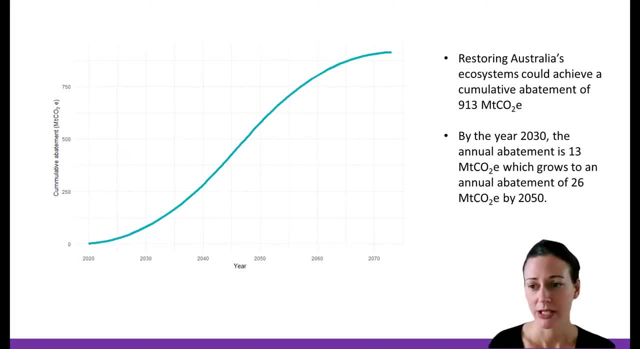 And we estimate that this would be sequestering a total of almost a billion tonnes of carbon dioxide equivalent And, under even current Australian policies, that could result in significant revenue being achieved from the abatement through carbon credits By 2030, the annual abatement, so the rise of this curve. 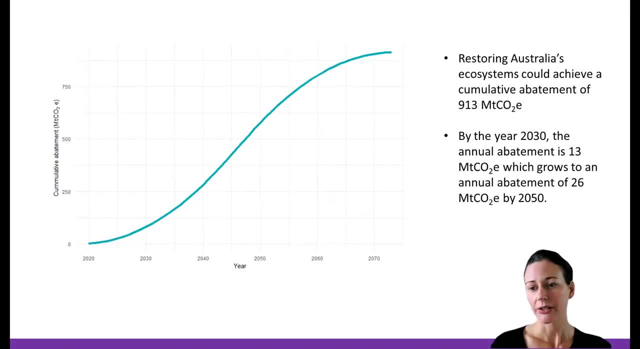 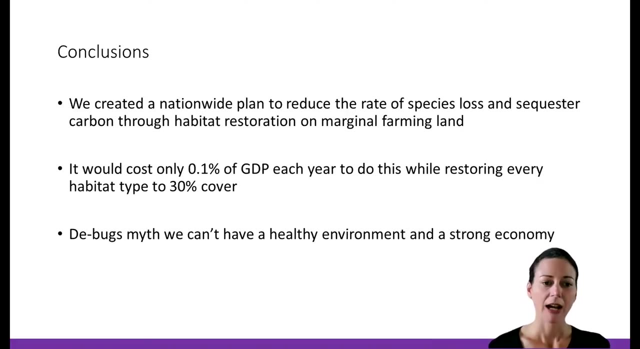 is at about 13 million tonnes of carbon dioxide equivalent, And by 2050, this grows to 26 million tonnes of carbon dioxide equivalent. So in this research, we created a national-wide plan to reduce the rate at which our species are being lost while sequestering carbon through. 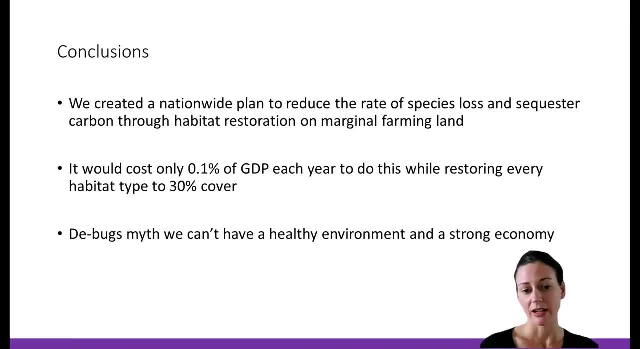 habitat restoration on marginal farming land and already established conservation areas. It would cost about 0.1% of GDP each year to do this And we believe that this deep bugs the myth that we can't have a healthy environment and a strong economy. Thank you. 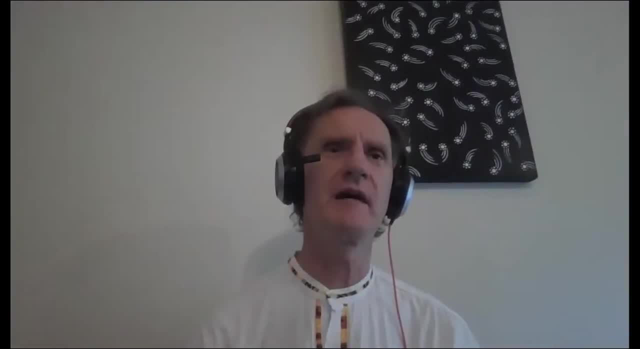 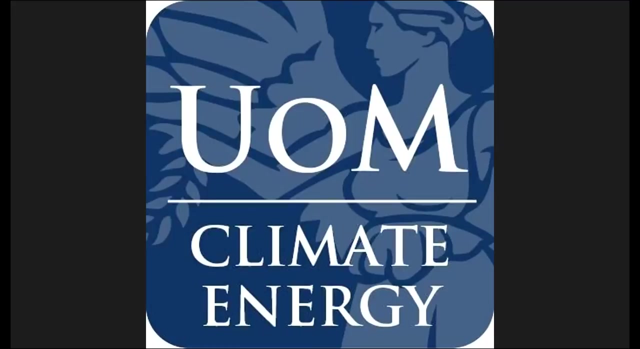 Great. Thanks very much. Now I'll hand over to Kate and Angela to moderate Q&A And I'll get myself back off video and unmute. Thank you, Peter. We've got time for a couple of questions, And so I'll start. 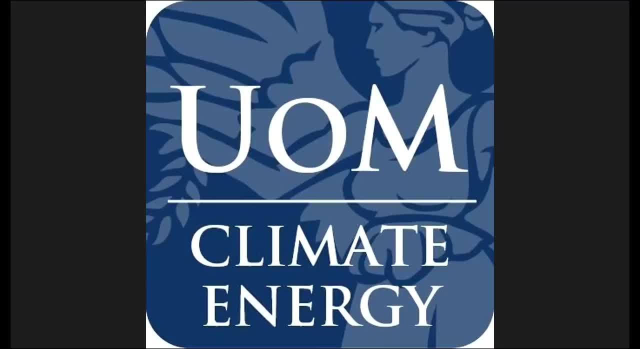 with a question from Malcolm McDonald, please. So give me a moment and I'll make it so that you can unmute yourself if you wanted to ask your question. Yes, I was interested in — I haven't got my question up — the question relates to the contribution of blue carbon. 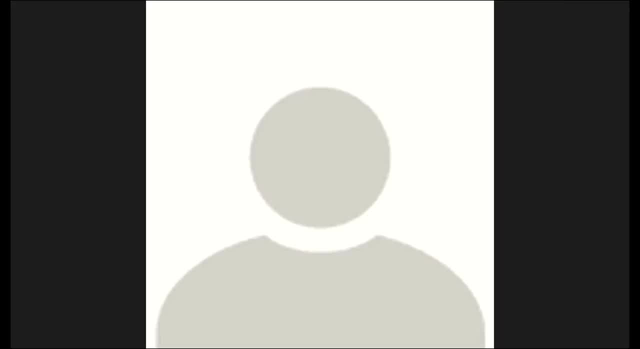 blue carbon sewer woody ammunition. Why does it make for less carbon? the contribution of blue carbon seagrasses, kelp and similar. with all the graphs that we saw, particularly the first one, how significant is that in terms of carbon uptake compared to land-based carbon? absorption? Thanks, Malcolm, I can take that question. So in terms of carbon uptake, coastal marine systems, seaweed, seagrass, salt marsh, etc. actually present a pretty small number. so while we're looking at, say, 5 to 10 gigatons of CO2. 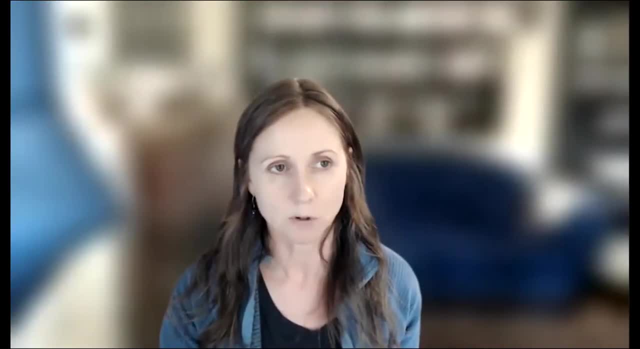 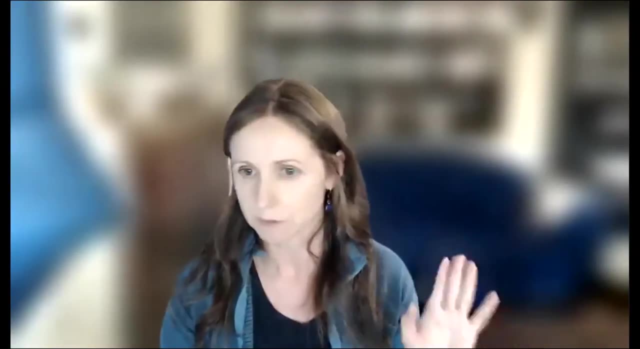 a year from terrestrial ecosystems it's more like 0.1% from marine ecosystems. that figure's not exactly right. that's kind of off the top of my head, but that's the order of magnitude. so it's a lot less. but that said, the coastal marine 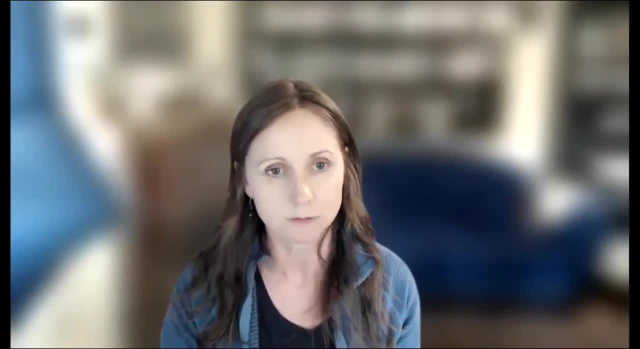 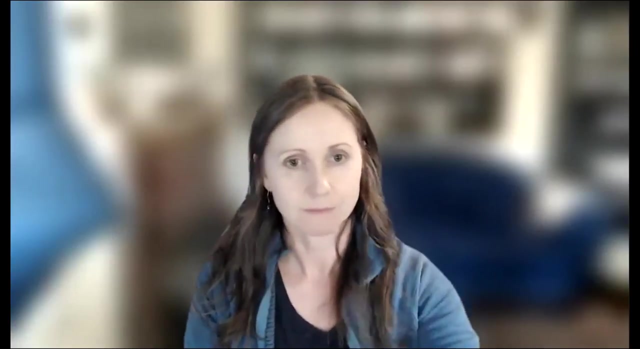 ecosystems are such important places in terms of biodiversity and ecosystem regulation, so they're really critical places to restore. they're just not significant carbon drawdown sites globally because they're small areas. Thank you, Thanks, Kate. Next we've got two questions from Roger East, please. so, Roger, 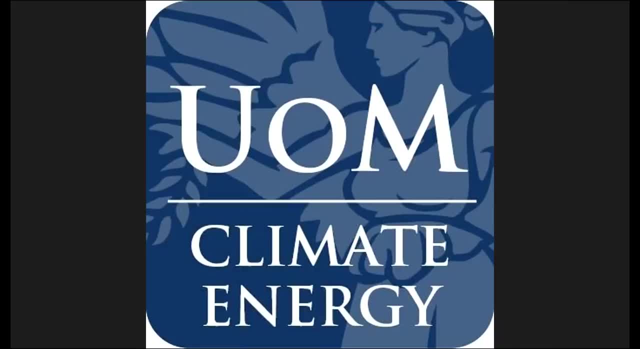 if you want to unmute yourself and ask your questions. Hello, look, thanks very much for that presentation. I guess the two questions I had is: how do we establish the amount of natural resources that we need to be able to use in the natural drawdown that's necessary by? 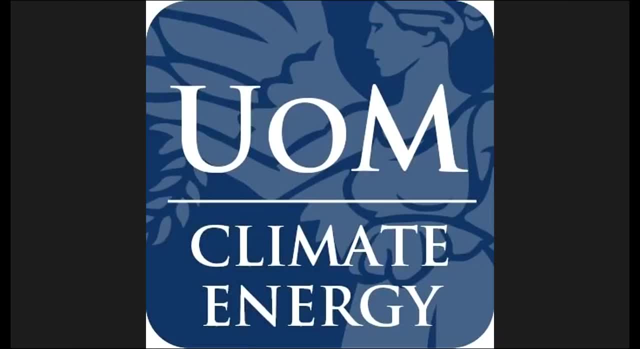 forestry and kelp forests and things like that to offset the natural emissions from volcanoes and rotting vegetation and stuff like that, and then determine what's left to offset the emissions from man, noting that historically the climate's been in balance and the temperature's been in. 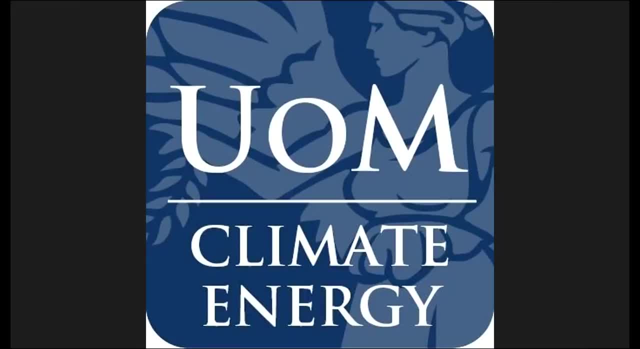 balance until we started to disrupt it. and the other question relates to using farmland and agricultural practices to sequester more soil carbon, and can that be done concurrently with increasing productivity of soil or is productivity naturally depleting soil? if we overgraze or whatever, does that naturally deplete soil? 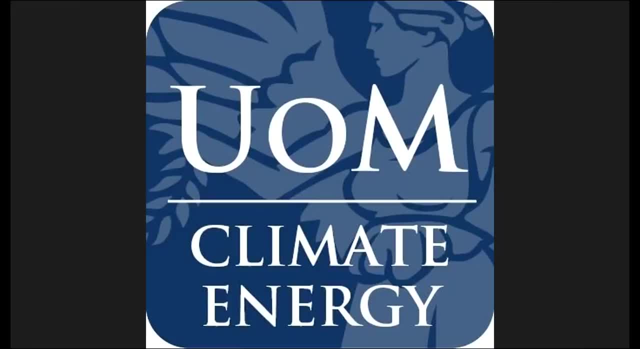 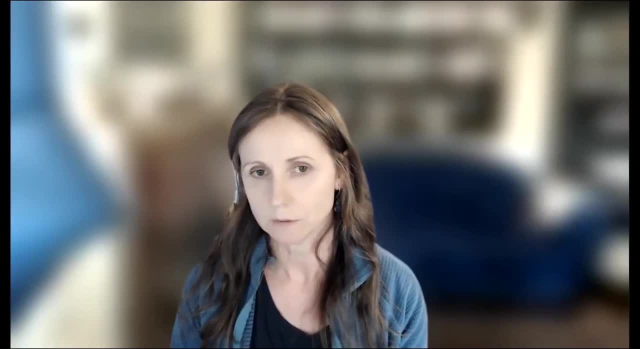 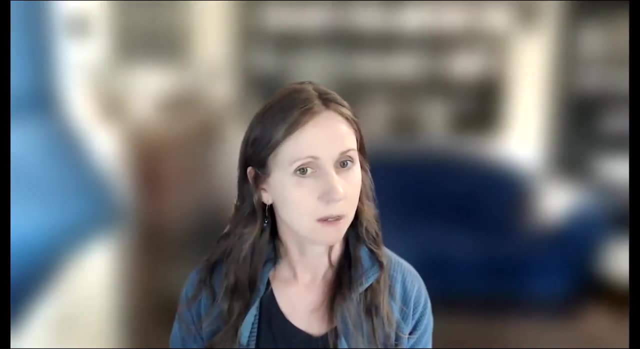 carbon. Thank you, I can start with that. I don't know if the others want to add something. So yeah, very good questions, Roger. In terms of sort of natural land use emissions, the land sector's always a bit complicated to think about. in terms. 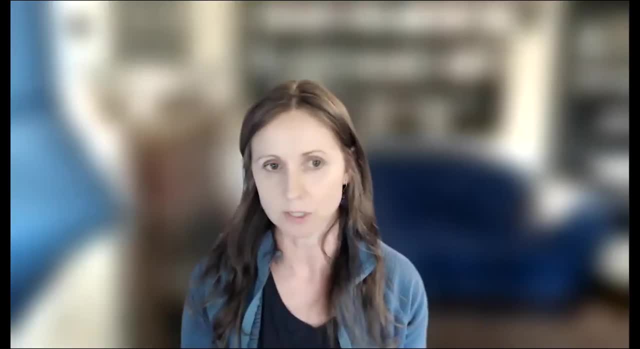 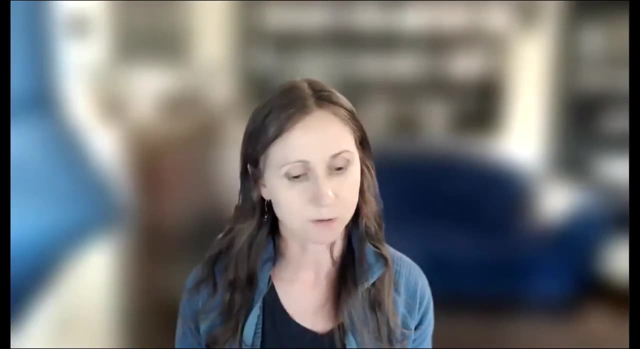 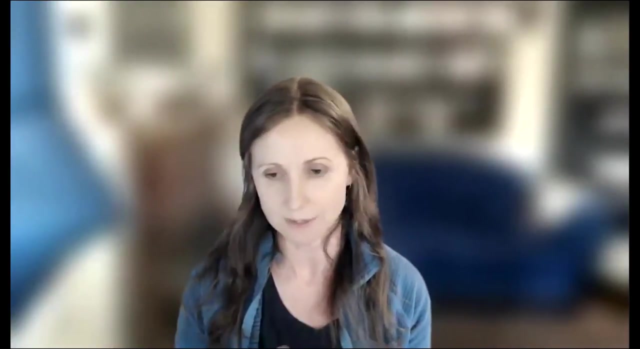 of mitigation, because we need to separate out the anthropogenic impacts of the land sector from natural, because land- actually land, and oceans sequester around half of anthropogenic emissions, so they're already taking up a lot of our emissions and so in that sense they're 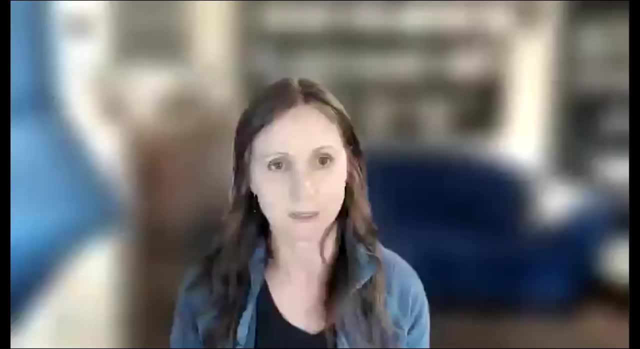 contributing to reducing warming on quite a large scale. but that's just the natural uptake of land and oceans. so we don't count that in the graphs and numbers I was showing you. we're not counting that what's called the, the residual land sink. it's a background. 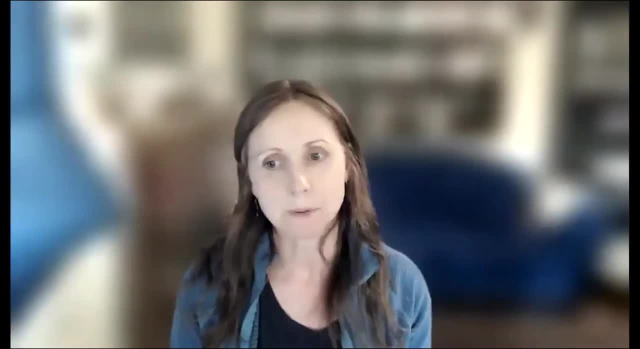 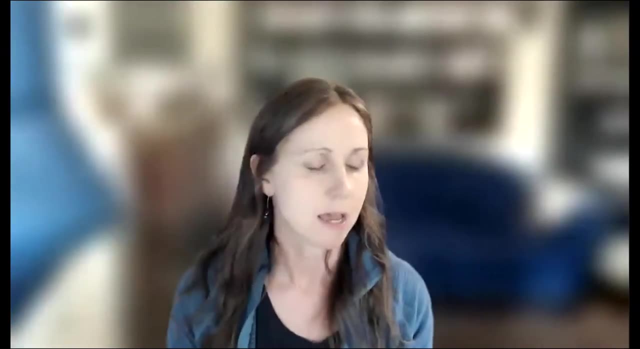 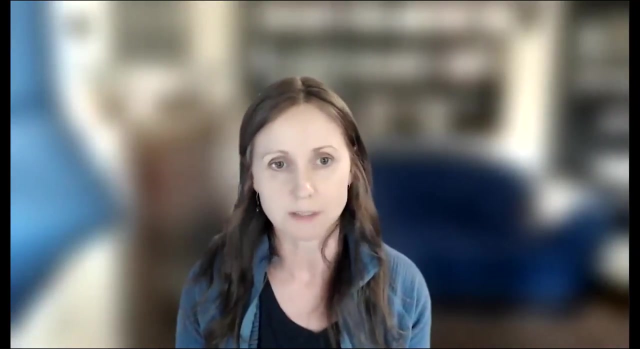 natural carbon cycle function. but another way- I find a clearer way to think about land and its role in climate change and its role in offsetting, say, natural emissions- is that we have depleted terrestrial carbon stocks and we could restore those depleted terrestrial carbon stocks, and so we're 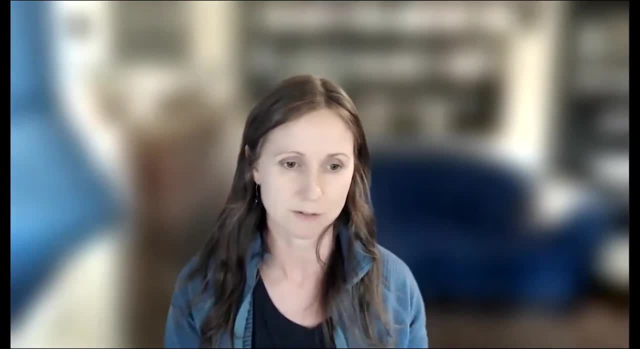 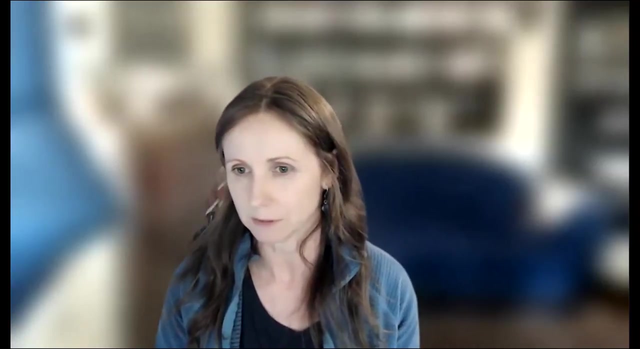 drawing down carbon that has been previously lost from the land. so it doesn't offset ongoing fossil fuel emissions but it can offset or restore emissions from the land sector, including natural processes such as methane. it's kind of a complicated topic. I hope that helps on the soil carbon. 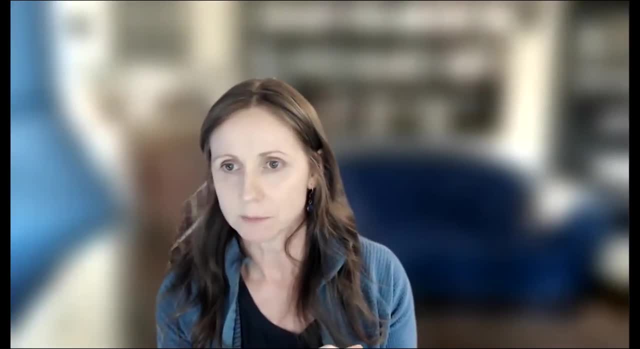 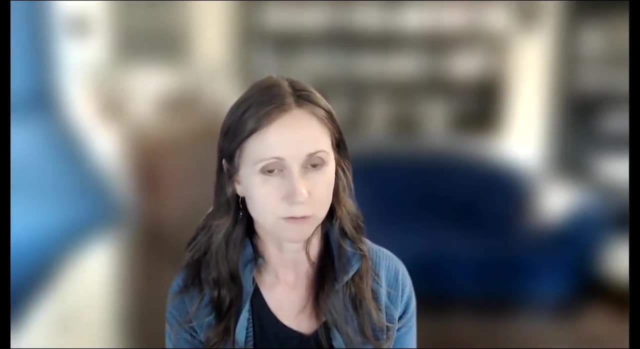 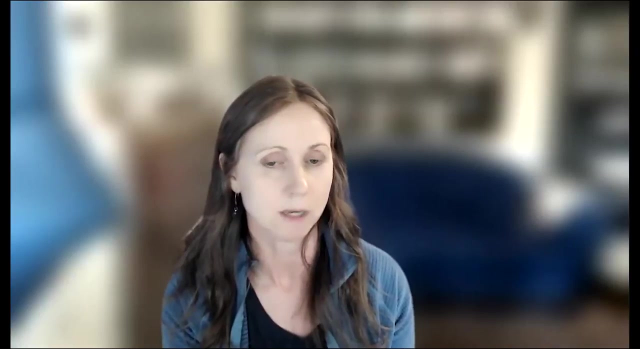 um. so the government's proposal to increase soil carbon and content- I mean increased soil carbon- increases farm productivity. it's very difficult to measure. it's also very difficult to keep carbon in the soil, particularly in drying climates, so this was actually a topic of our seminar last week. 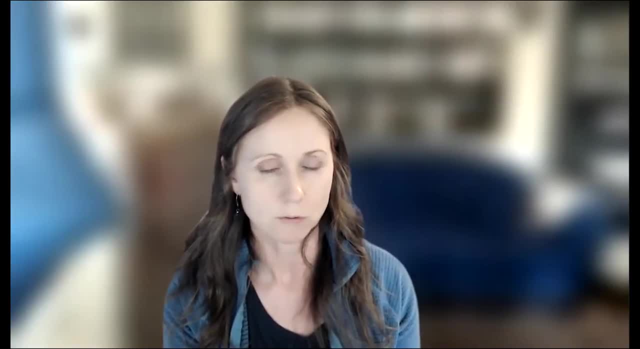 Rachelle Meyer has done a lot of work on this. so many the government's estimates for soil carbon mitigation are probably over inflated, but at the same time it's an important strategy for farmers for productivity increase. I don't know if others want to add to those answers. 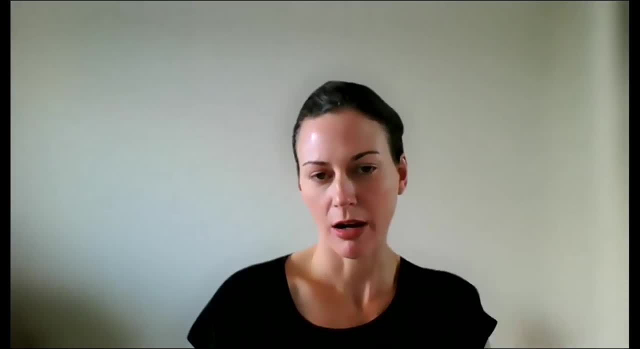 I agree with that. um, not myself, but one of the members who went with fruit. I've had a discussion with about the soil carbon specifically in Australia, and that the numbers, even if they are inflated, they're- um, they're actually quite small in terms of what impact that. 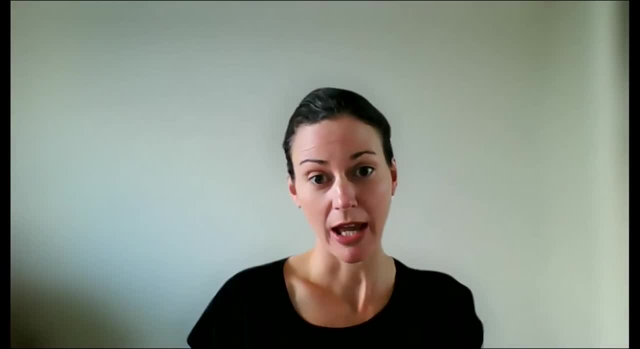 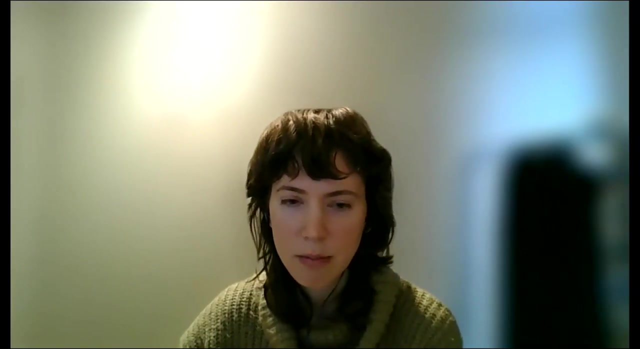 they will have in terms of compared to how much we're emitting. so, as much as it can be a strategy, it's not going to significantly offset how much we're emitting. maybe I can just add, at least for the European Union perspective, the land use sink, which is mainly 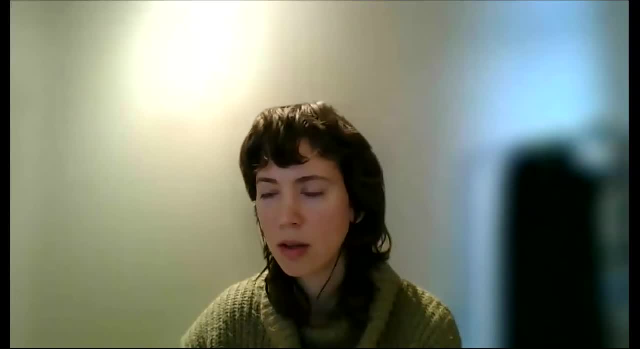 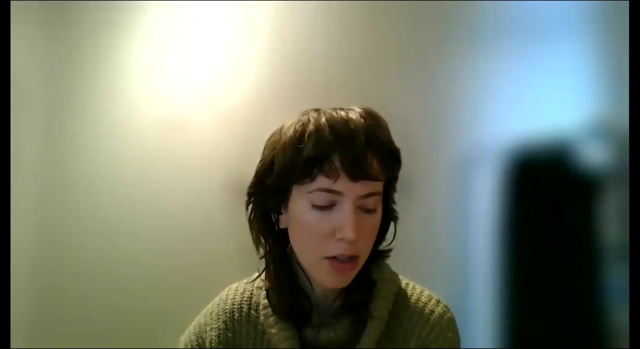 forests is the equivalent to about eight percent of the overall fossil fuel emissions coming from the European Union, so it's definitely not a viable means of offsetting what's happening in terms of fossil fuel production and the way that the European Union has gone about it not perfectly. 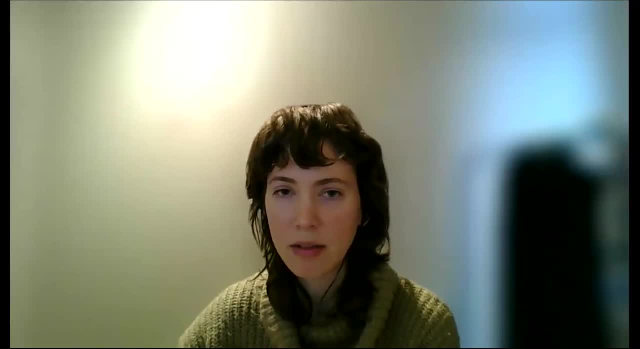 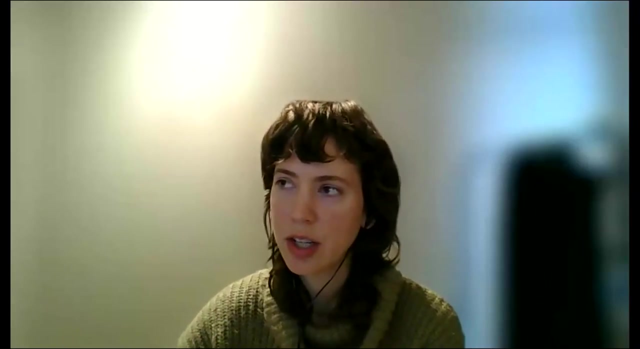 is to attempt to establish a limit of the contribution of the land use sector to the overall European Union targets to reduce emissions. so there's an attempt to sort of have pillars where land use is treated on one side and where emissions reductions are treated on the other side. 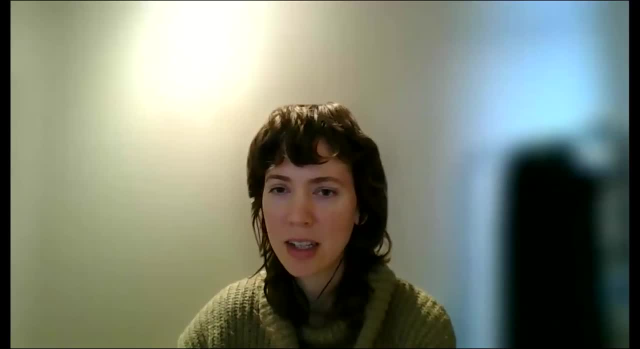 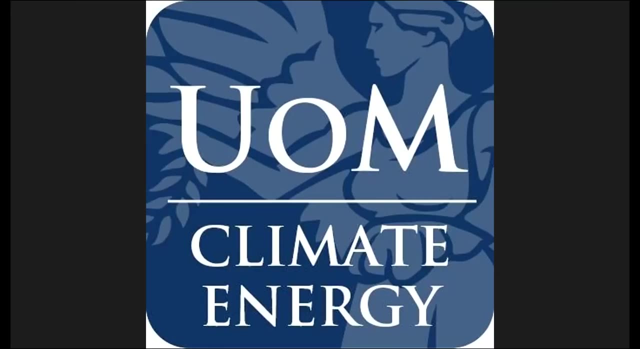 so yeah, but other than that, I agree with what Kate and Bonnie have added. Thank you all. the next question is from Jeff. so, Jeff, I'll ask you to unmute yourself, and if anybody else has questions, do either pop them in the Q&A or raise your hand and we'll get to you shortly. 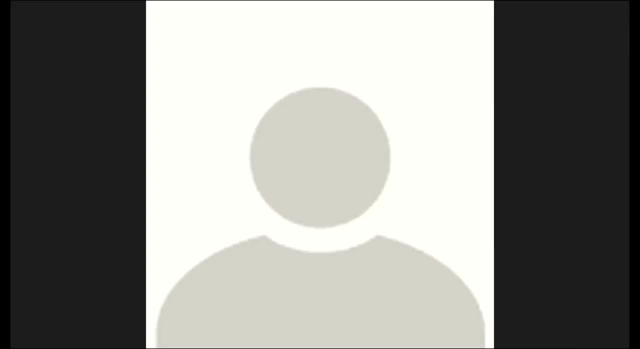 I was interested and Kate answered the difference between silvopasture and agroforestry in my chat and that was interesting, that one was on cropland and one was on pasture land. so thank you for that, Kate. a question for Bonnie: when you were calculating, 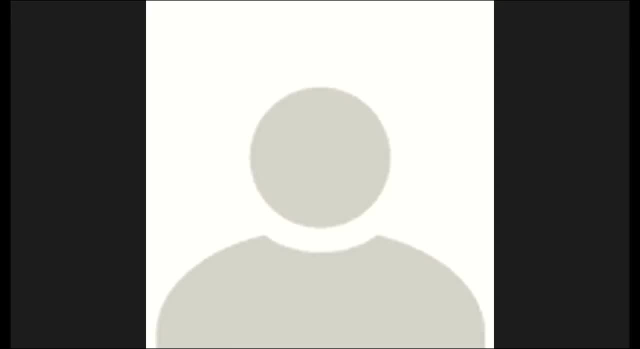 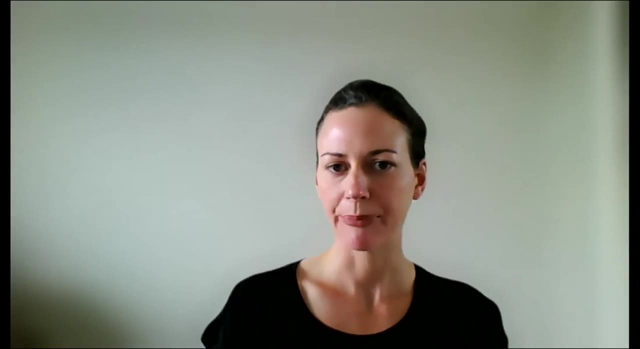 the NPV of the costs. what rate of value for the carbon credits did you use? can I ask? because you came up with a 41 billion NPV? I think was the yeah, so the cost that I'm presenting is how much it would cost the direct. 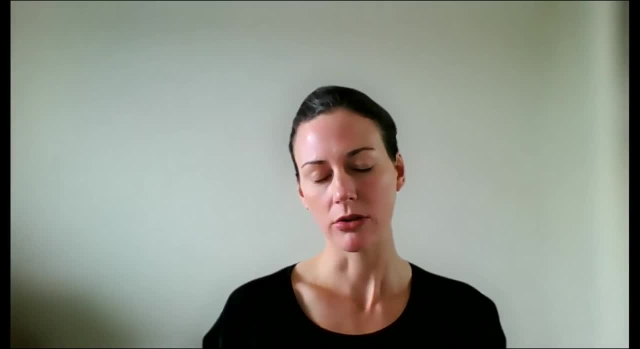 restoration costs and not how much revenue, but, sorry, the net present value of the cost. that was the direct restoration cost, the stewardship cost and the management fee put together. however, I didn't present it, but in the research we also calculated the expected revenue that could be received now. 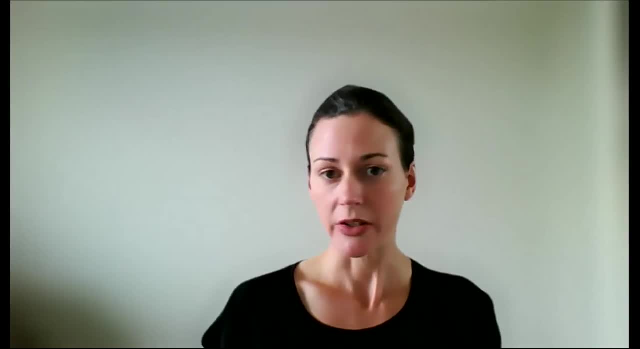 obviously, over time, things are going to change, and so these are just assumptions. but if we were able to, if all the all the carbon abated on the private land was able to be sold at the time in which it's being sequestered, so it is over. a 55 year period. we assumed $15 a ton right now and that, going up at 10% per annum, that the actual revenue would be in the order of about $46 billion net present value. so it's actually more revenue than the cost to restore the land. as I said, there's a that's over a very long time period and things will change, but yeah, the profits are significant. yeah, so it would be offset, which I think is good. I think the current spot price is about $56 a ton in Australia at the moment. 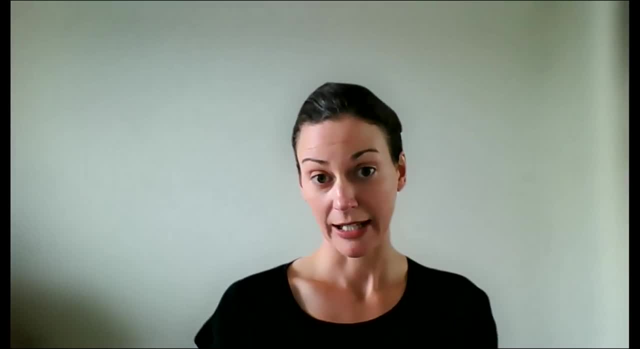 yeah, so it's gone up significantly since when I started that research. yeah, and it's looking like it's going to keep growing up. however, as I said, you have to have some assumptions, but it is going to change over that huge time period- wonderful. thank you, Bonnie. 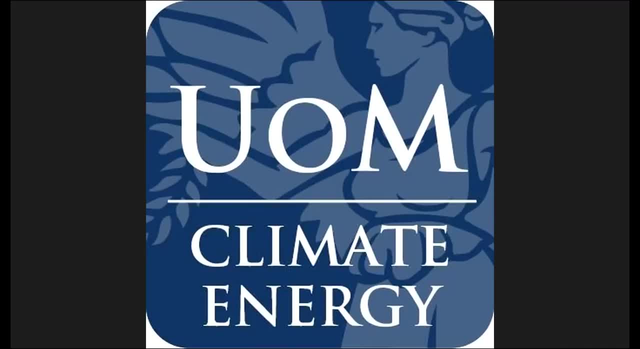 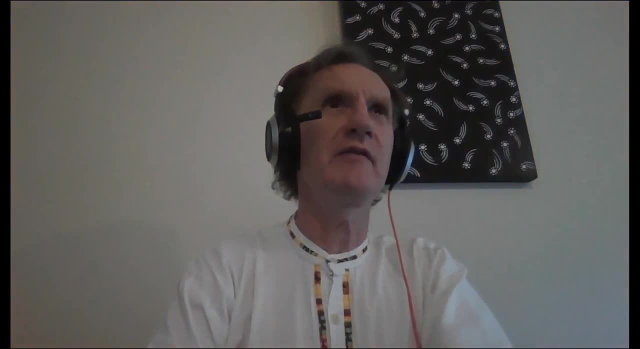 there's no further questions. so I'll hand back to Peter, as we're right on time for any closing comments, and I'll just unmute myself and get myself back on video. so thanks very much to the three of you. I've got several questions. I'll probably 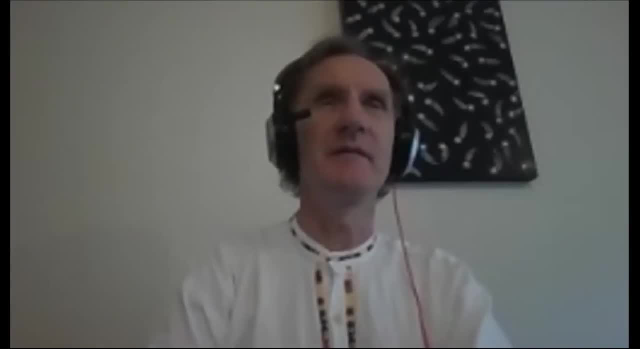 take up separately with you afterwards as well, which probably indicates that at least I found that a really fascinating range of insights into the problems and possibilities and it it really does sound as though thinking about this as a carbon solution is useful, but it's far more powerful when we 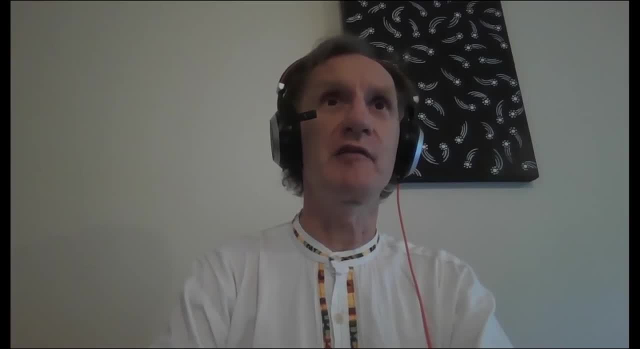 manage to consider the full range of environmental consequences of actually dealing with restoration and protection of landscapes, and that's very encouraging. in some sense not hugely surprising, but actually being able to put values on those things really strengthens the arguments clearly. so thanks again to the speakers and to all for 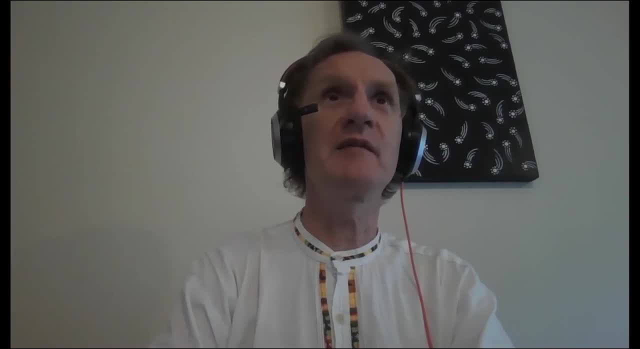 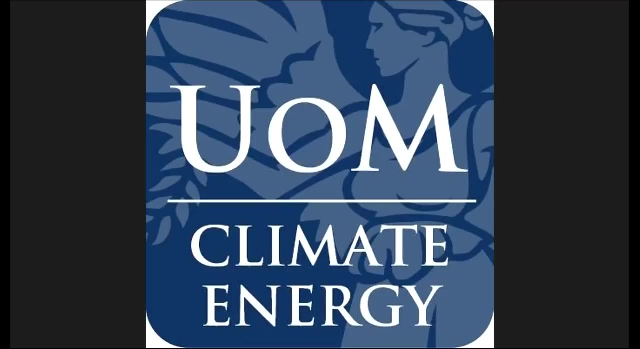 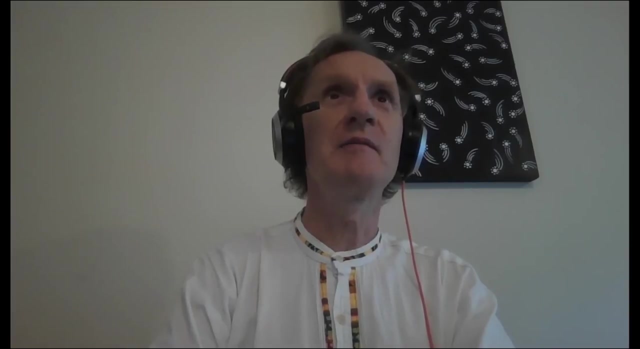 coming note that we have a seminar coming up again in- I think it's a week, is it Angela? that's correct- next Tuesday same time. so next Tuesday, same time, major change of theme in the way that the kind of breadth of this topic demands. we'll be looking.